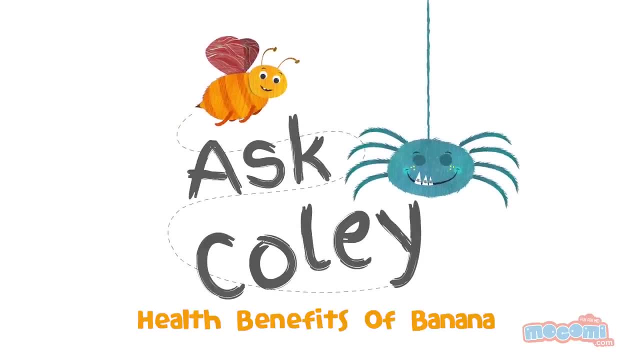 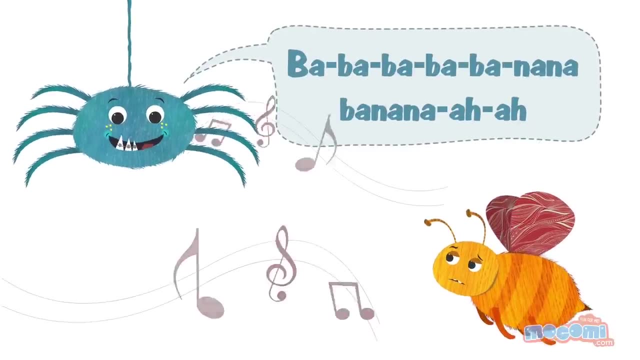 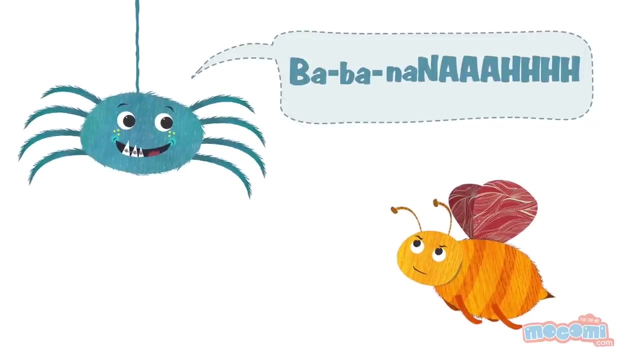 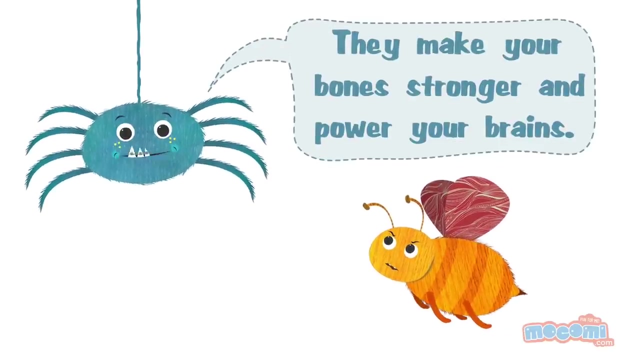 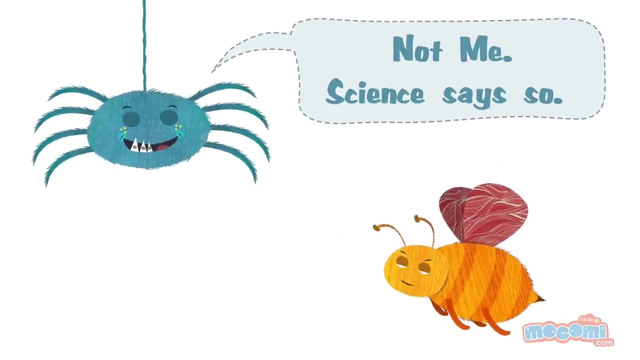 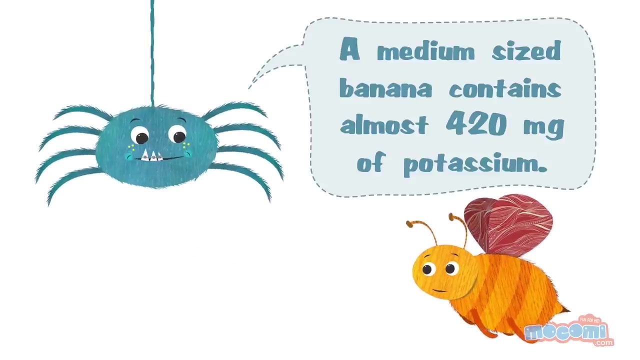 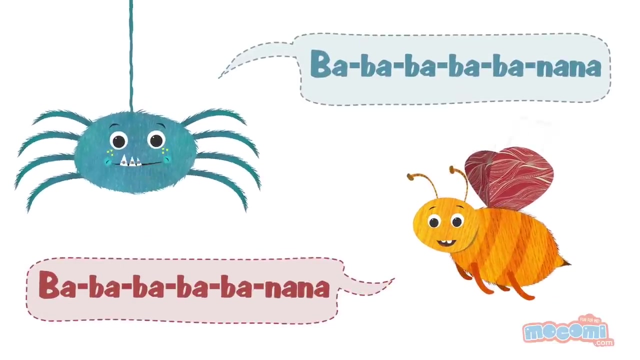 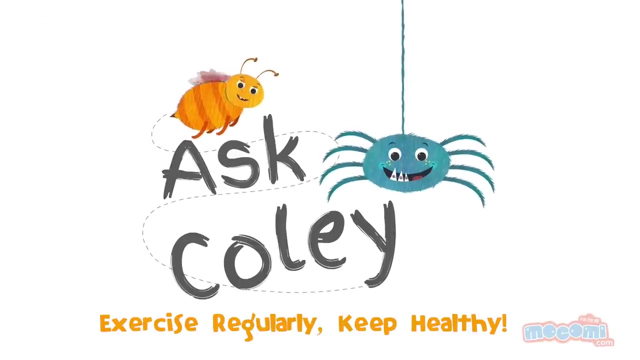 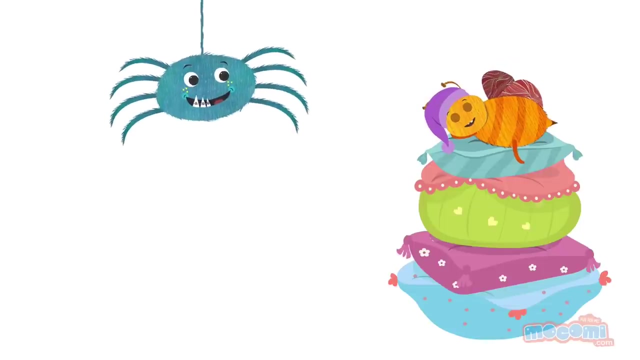 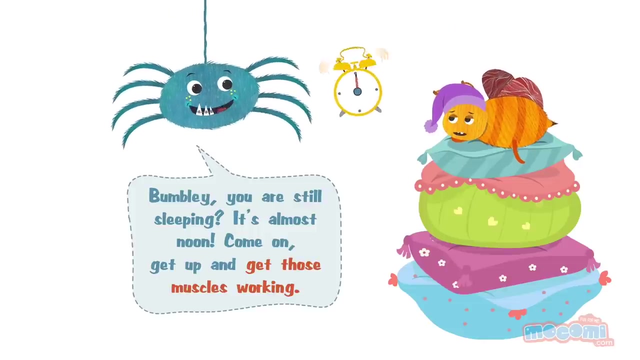 Thank you for watching, Not me. Science says so. A medium sized banana contains almost 420 mg of potassium. Wow, Now I think I love bananas too. Bumbley, you are still sleeping. It's almost noon. Come on, get up and get those muscles working. 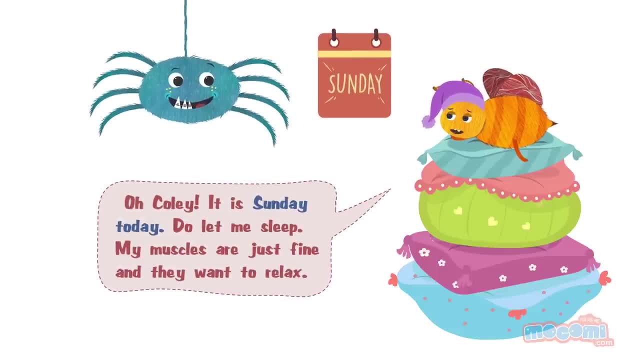 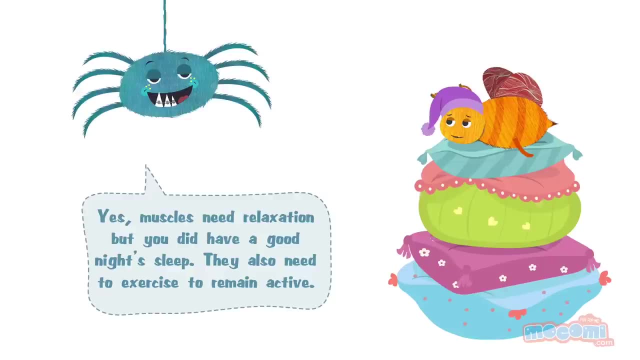 Oh, Coolie, it is Sunday today. Do let me sleep. My muscles are just fine and they want to relax. Yes, muscles need relaxation, But you did have a good night's sleep. They also need to exercise to remain active. 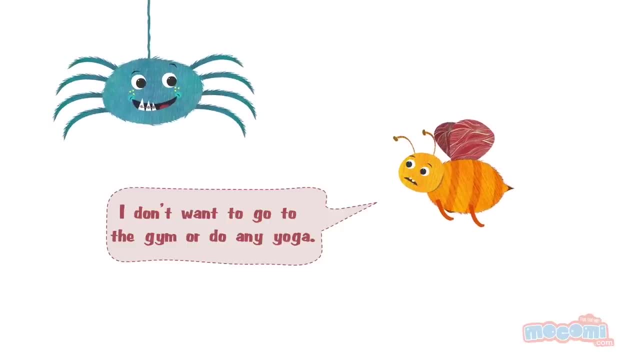 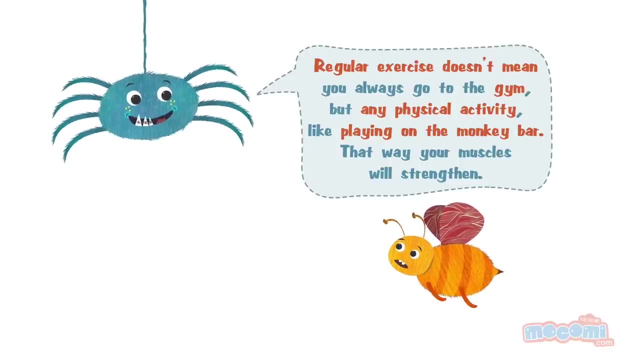 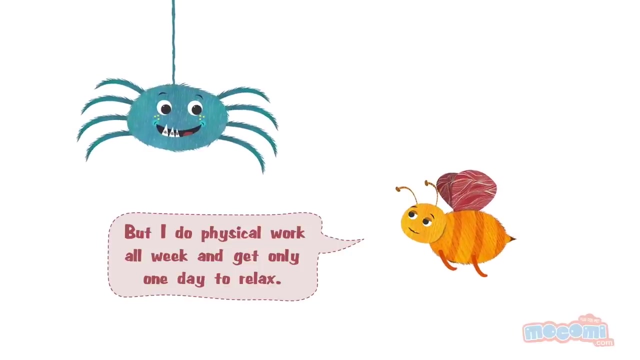 I don't want to go to the gym or do any yoga. Regular exercise doesn't mean you always go to the gym, But any physical activity like playing on the monkey bar. That way your muscles will strengthen. But I do physical work all week and get only one day to relax. 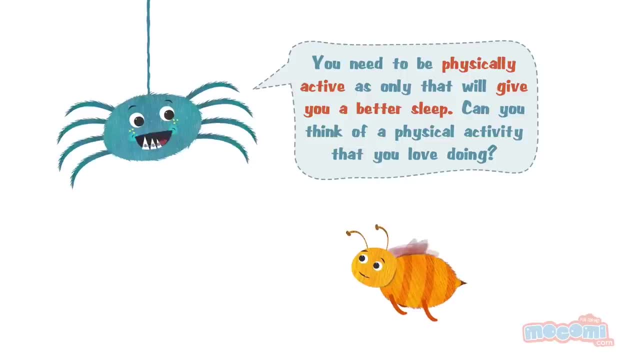 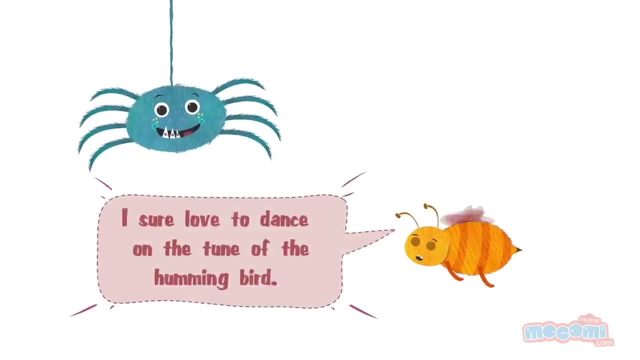 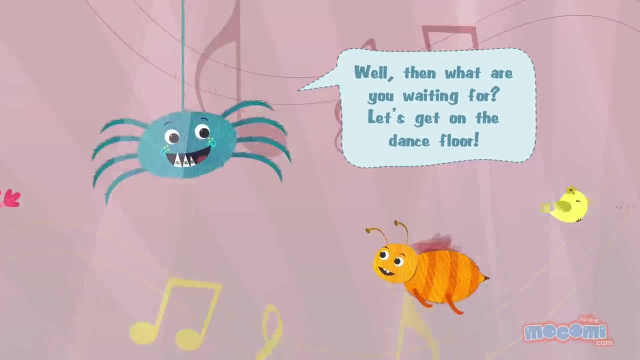 You need to be physically active, As only that will give you better sleep. Can you think of a physical activity that you love doing? I sure love to dance on the tune of the hummingbird. Well then, what are you waiting for? Let's get on the dance floor. 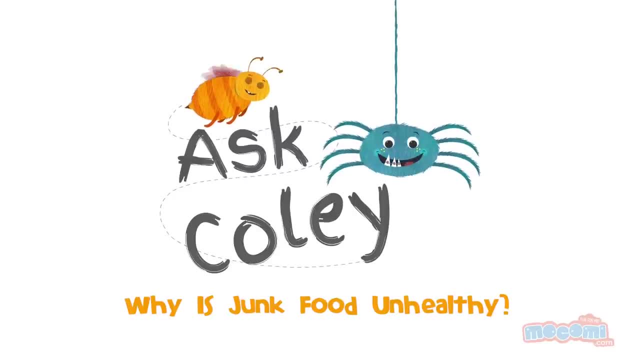 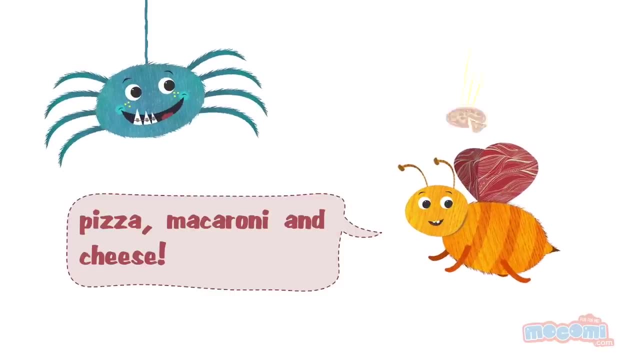 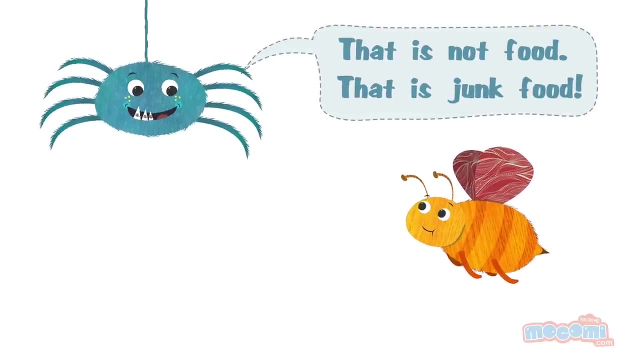 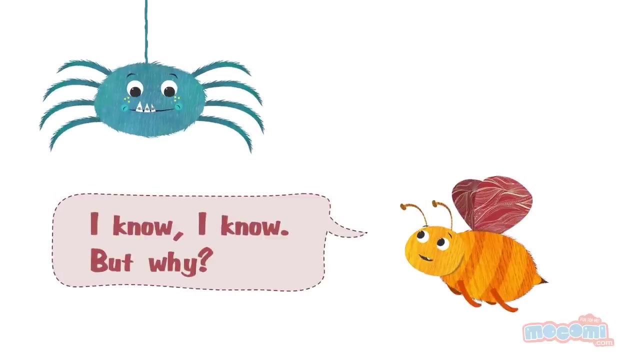 Music, A dollop of ice cream, a piece of chocolate, Pizza, macaroni cheese, Pizza, macaroni cheese and cheese. oh how I love food. that is not food, that is junk food. and you know that junk food is unhealthy. right, I know, I know, but why? I mean? how can something? 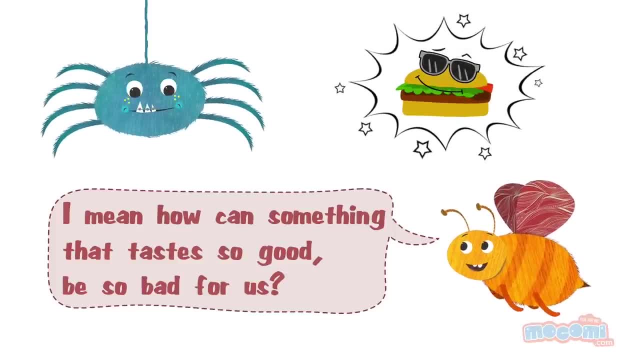 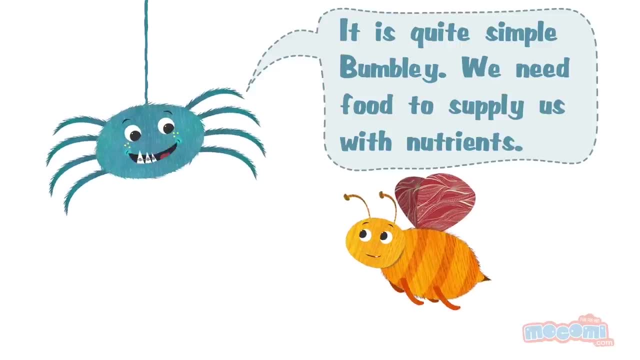 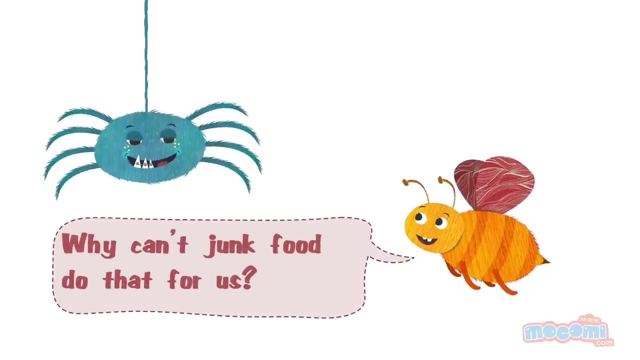 that tastes so good be so bad for us? it is quite simple, Bumbley: we need food to supply us with nutrients, nutrients which are used to build our body and fuel it. why can't junk food do that for us? because junk food doesn't have enough. 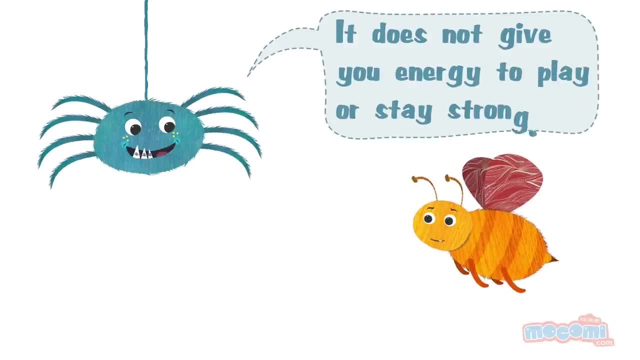 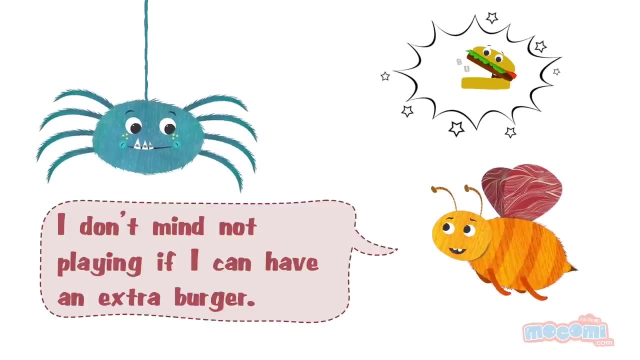 nutrients in it. it does not give you energy to play or stay strong. I don't mind playing if I can have an extra burger. really, you prefer a burger. I don't mind playing if I can have an extra burger. really, you prefer a burger. I don't mind playing if I can have an extra burger- really you prefer. 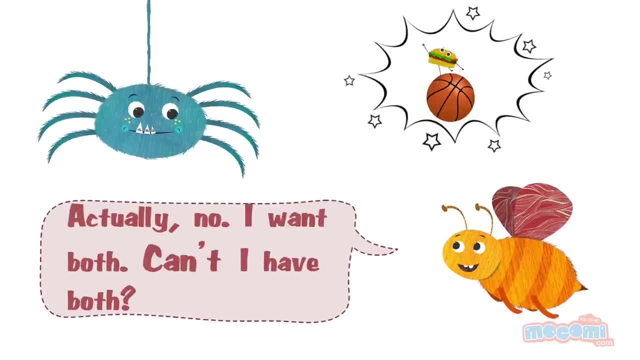 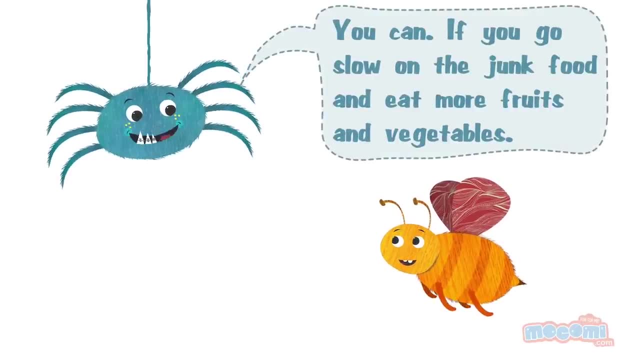 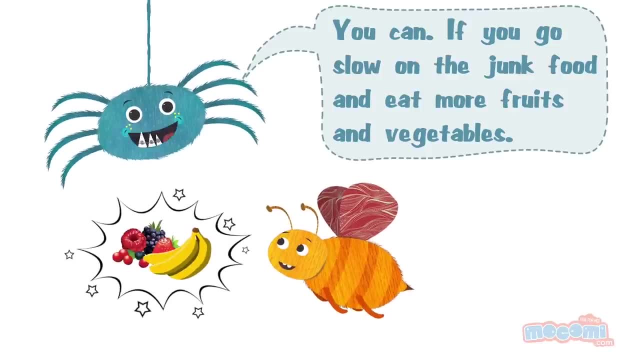 both can't, I have both. you can. if you go both can't, I have both. you can. if you go slow on the junk food and eat more slow on the junk food and eat more slow on the junk food and eat more fruits and vegetables. that way you are. 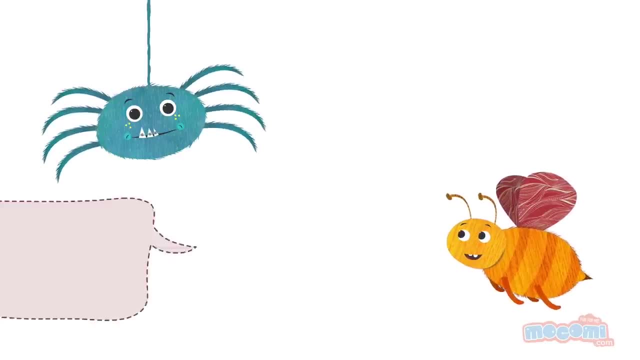 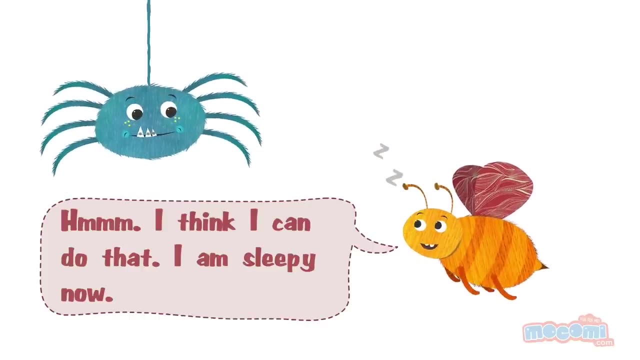 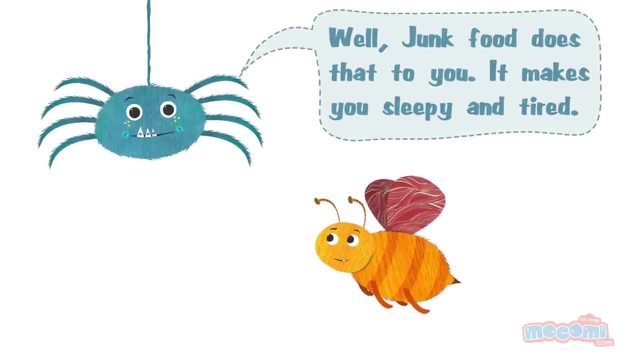 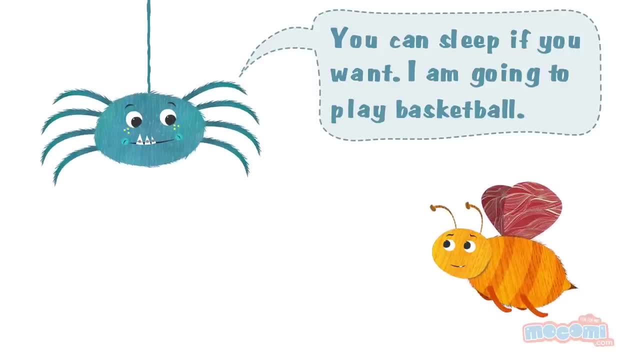 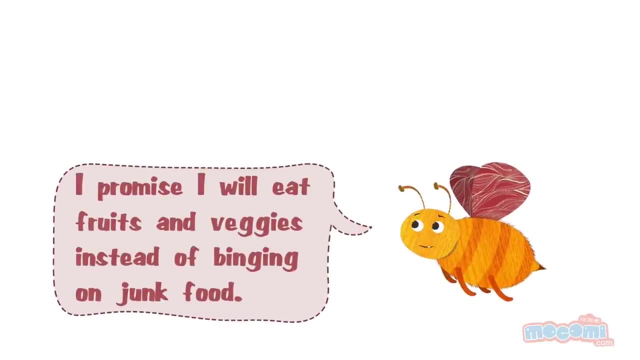 you sleepy and tired, you can sleep. if you sleepy and tired, you can sleep. if you want, I'm gonna play basketball. no, you want, I'm gonna play basketball. no, you want, I'm gonna play basketball. no, wait for me, I do want to play, I promise. wait for me, I do want to play, I promise. 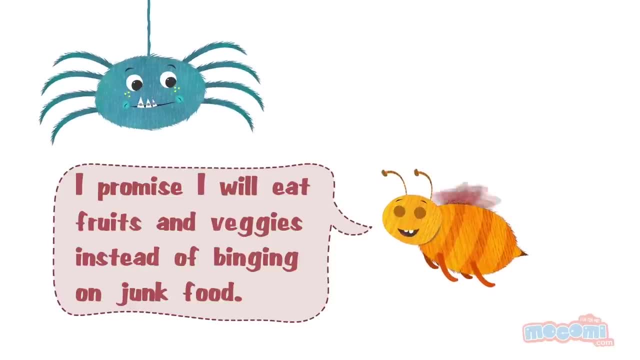 wait for me. I do want to play. I promise I will eat fruits and veggies instead of. I will eat fruits and veggies instead of. I will eat fruits and veggies instead of. pinging on junk food. playing is a lot. pinging on junk food playing is a lot. 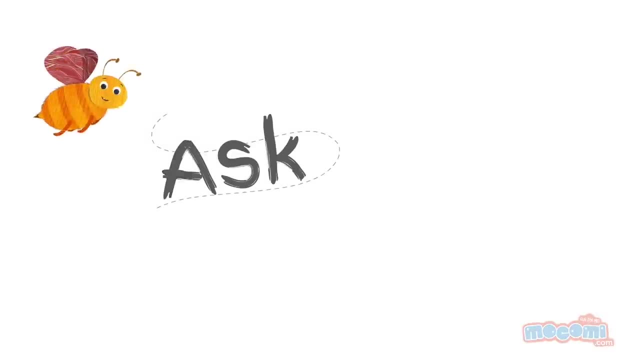 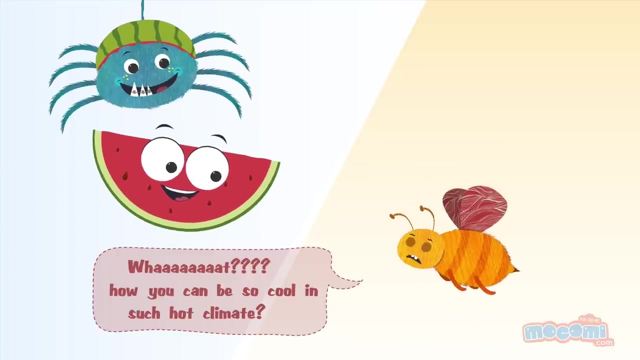 pinging on junk food. playing is a lot more fun, more fun, more fun. how can you be so cool in such hot? how can you be so cool in such hot? how can you be so cool in such hot climate? it's because of my friend climate. it's because of my friend. 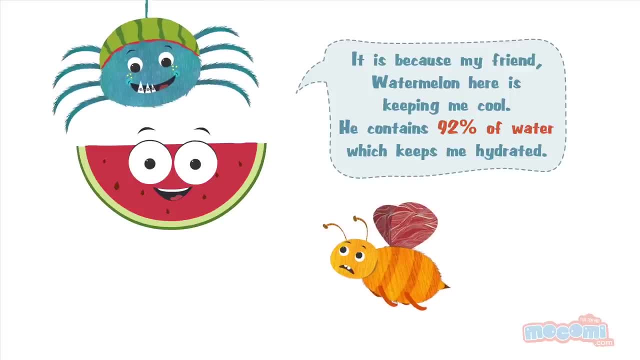 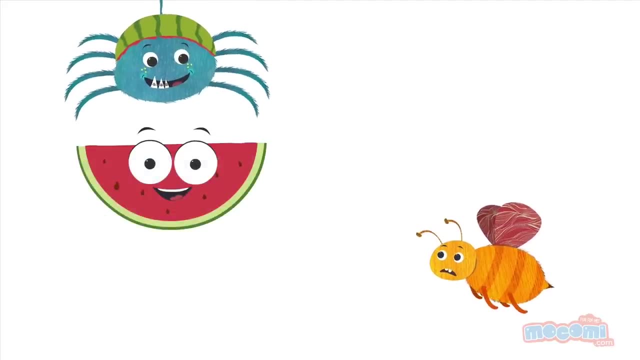 climate. it's because of my friend watermelon here is keeping me cool. he watermelon here is keeping me cool. he watermelon here is keeping me cool. he contains 92% of water which keeps me. contains 92% of water which keeps me. contains 92% of water which keeps me hydrated. 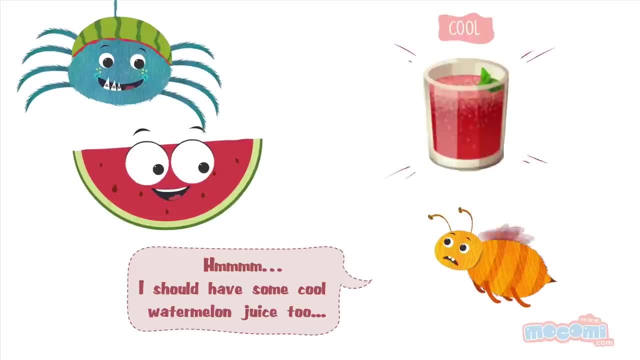 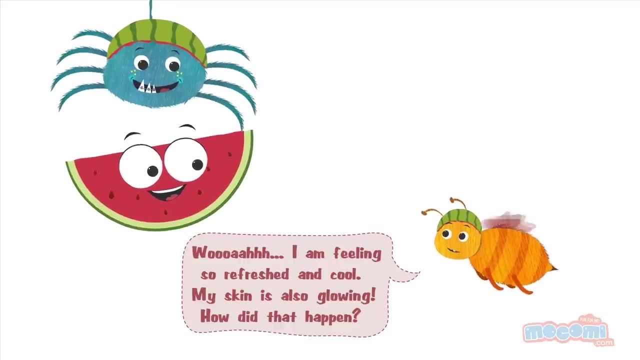 hydrated, hydrated. hmm, I should have some cool watermelon. hmm, I should have some cool watermelon. hmm, I should have some cool watermelon juice too. wow, I'm feeling so refreshed juice too: wow, I'm feeling so refreshed juice too: wow, I'm feeling so refreshed and so cool. my skin is also glowing. how 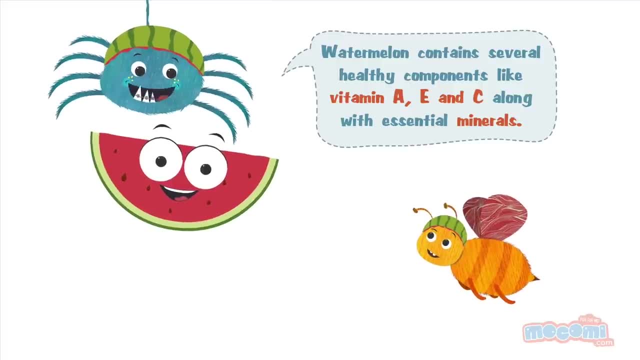 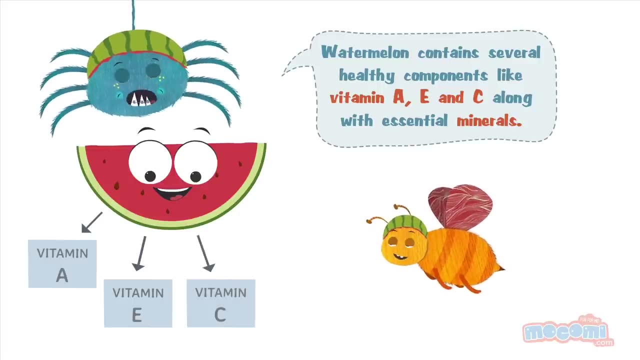 and so cool my skin is also glowing. how and so cool my skin is also glowing. how did this happen? watermelon contains- did this happen? watermelon contains- did this happen? watermelon contains several healthy components like vitamin, several healthy components like vitamin, several healthy components like vitamin A, E and C, along with essential minerals. 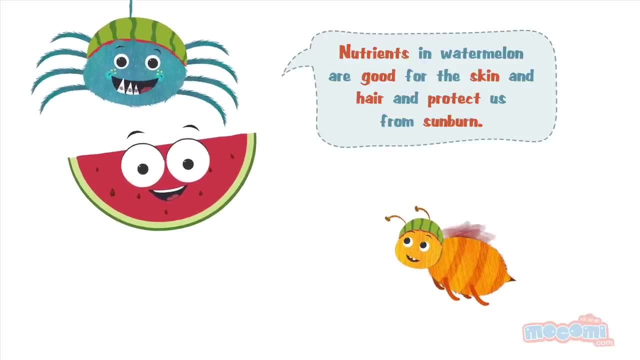 A, E and C, along with essential minerals- A, E and C, along with essential minerals. nutrients in watermelon are good for. the nutrients in watermelon are good for. the nutrients in watermelon are good for the skin and hair and protect us from sunburns- skin and hair and protect us from sunburns. 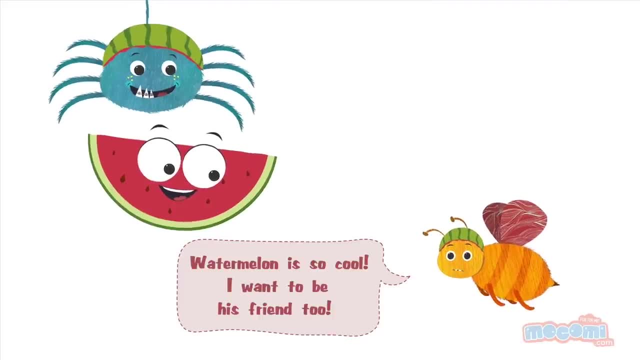 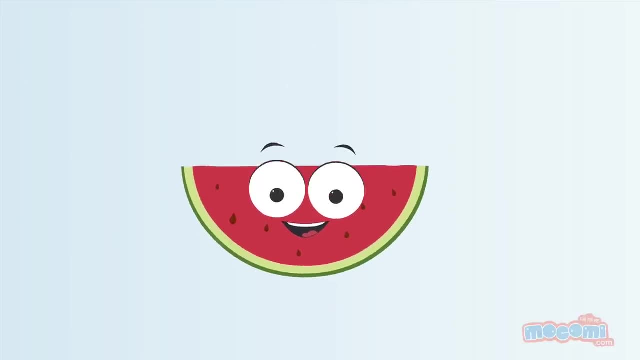 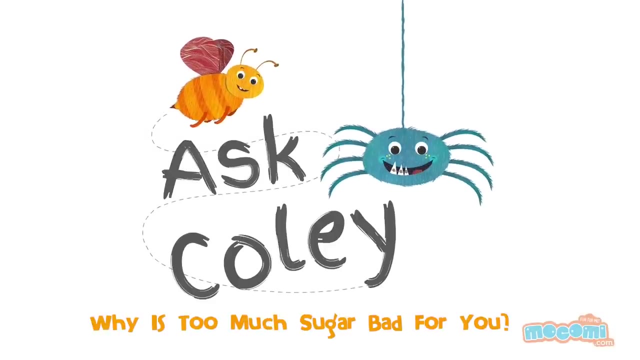 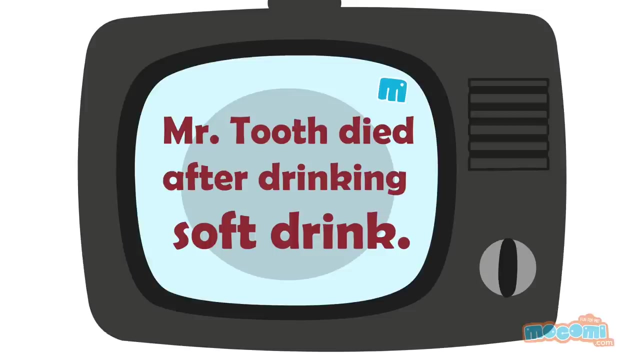 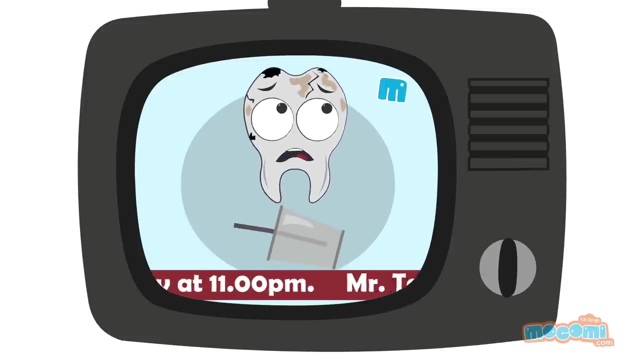 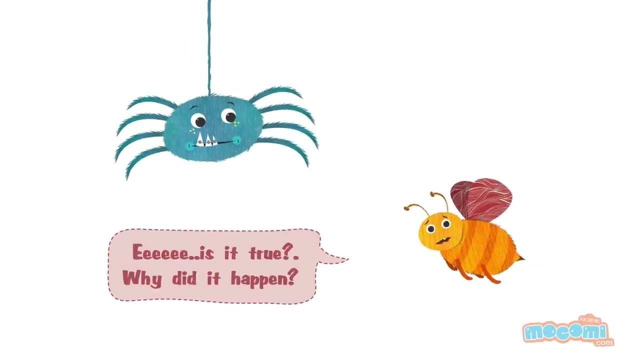 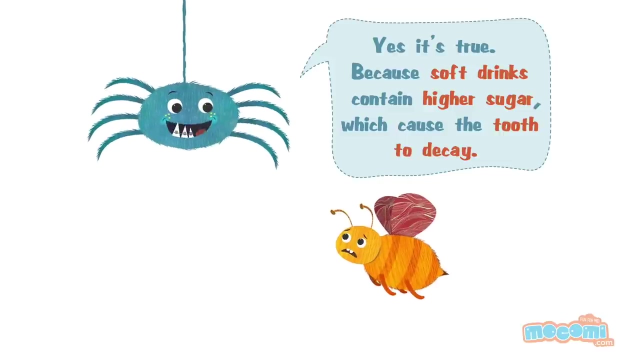 skin and hair and protect us from sunburns. watermelon is so cool, I wanna be its. watermelon is so cool, I wanna be its. watermelon is so cool, I wanna be its friend too. friend too, friend too. Yes, it's true, because soft drinks contain higher sugar, which cause the tooth to decay. 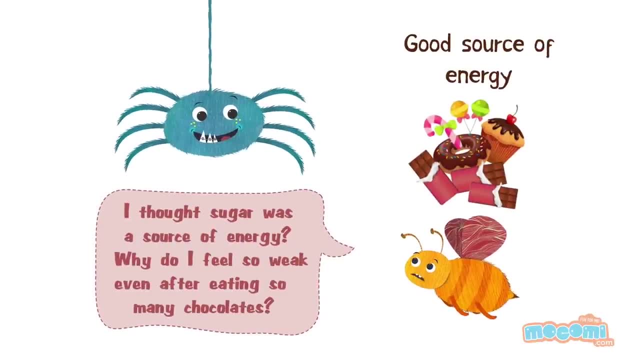 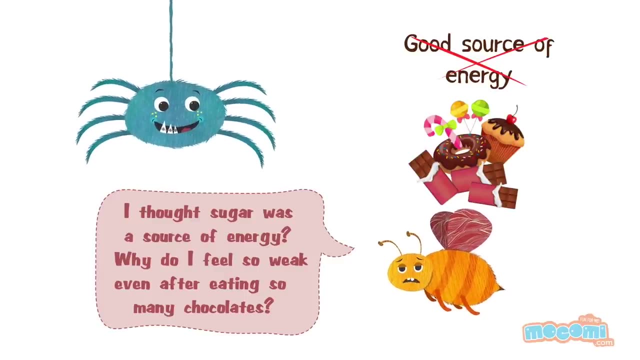 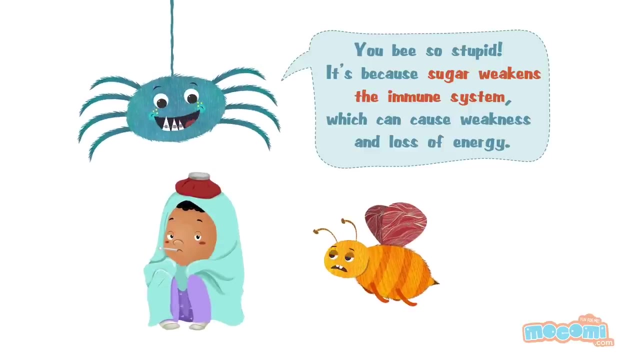 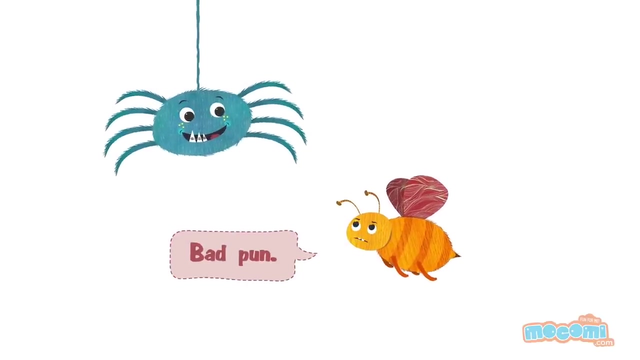 I thought sugar was a source of energy. Why do I feel so weak, even after eating so many chocolates? You be so stupid. It's because sugar weakens the immune system, which can cause weakness and loss of energy. Bad one, My legs are paining. 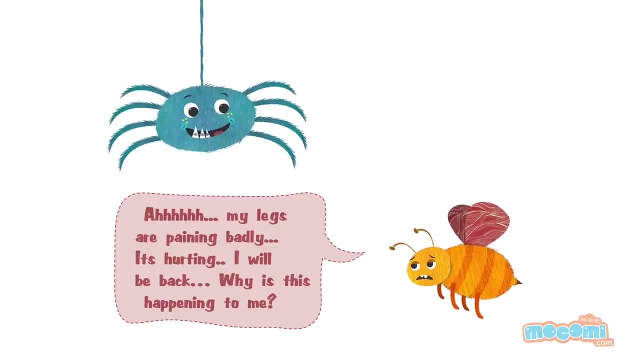 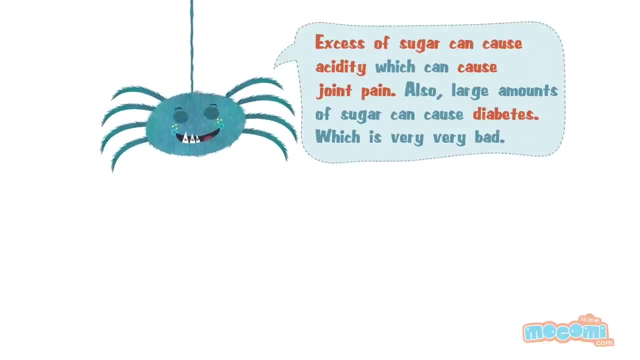 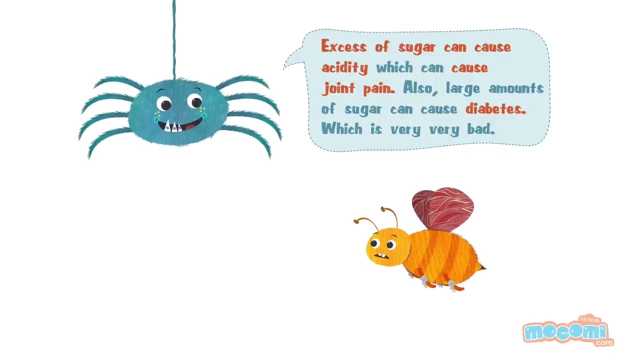 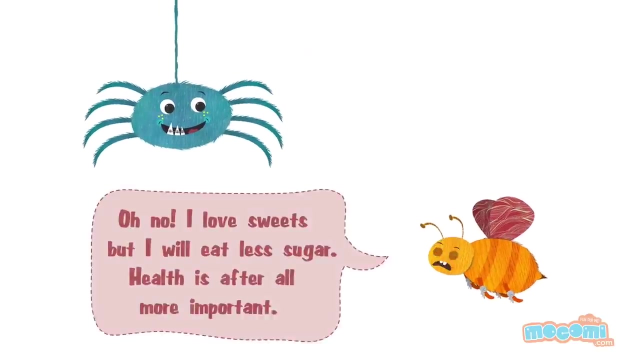 It's hurting. I will be back. Why is this happening to me? Excess of sugar can cause acidity, which can cause joint pain. Also, large amounts of sugar can cause diabetes, which is very, very bad. Oh no, I love sweets, But I will eat less sugar. 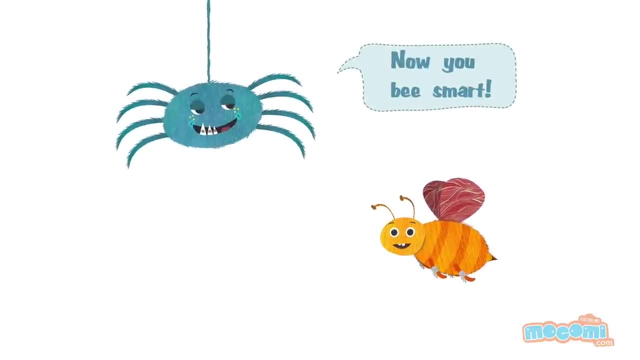 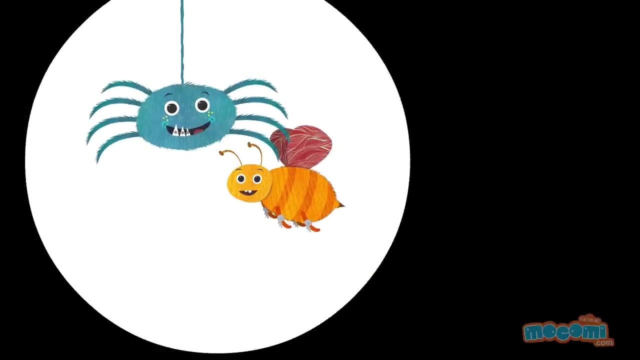 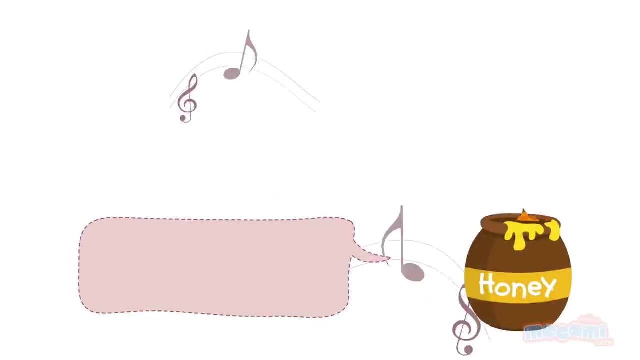 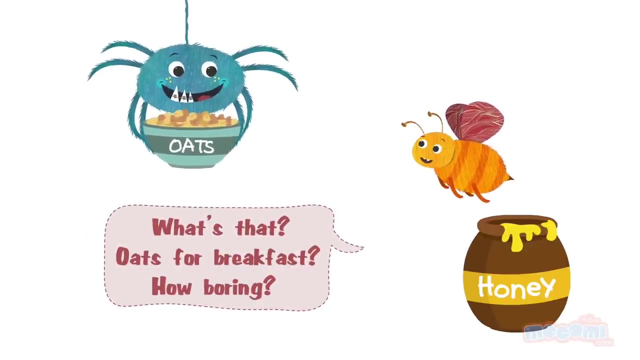 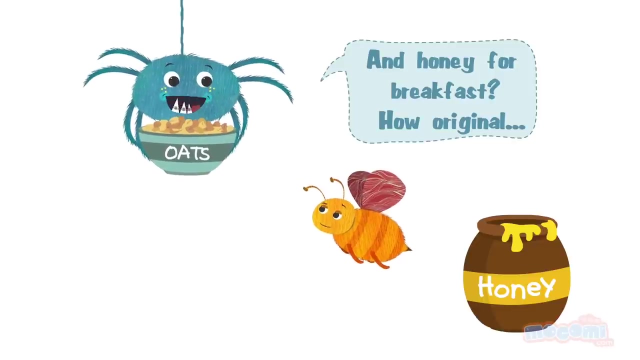 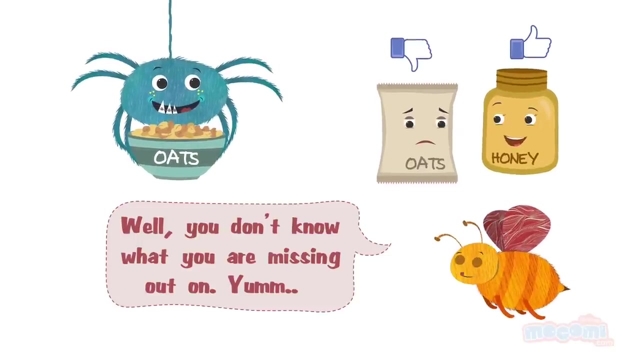 Health is, after all, more important. Now you be smart. Why another bad pun? Honey, oh honey, how I love my honey. What's that? Oats for breakfast, How boring, And honey for breakfast, How original. Well, you don't know what you're missing out on. 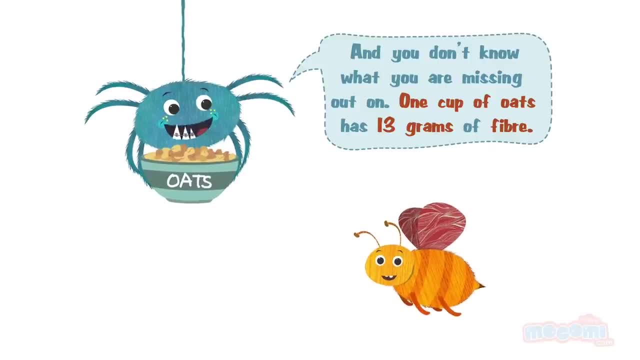 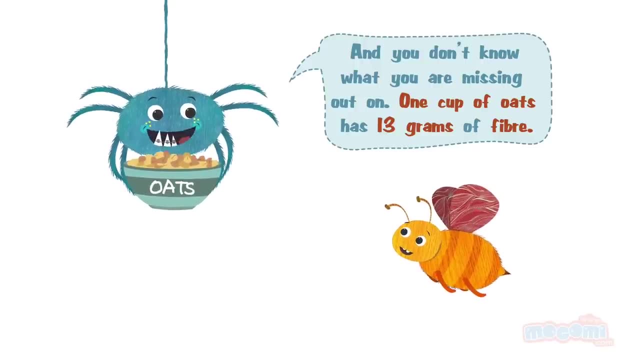 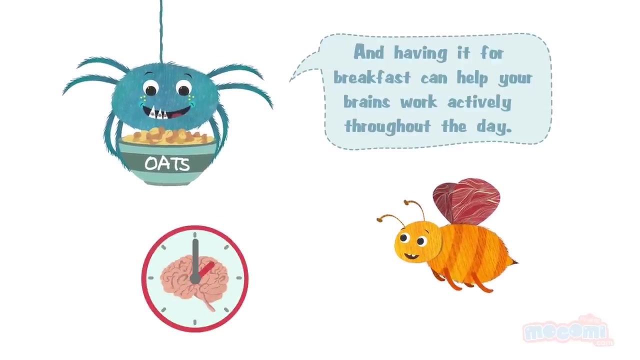 Yummm, And don't you know what you're missing out on? One cup of oats has 13 grams of fibre, and having it for breakfast can help your brains work actively throughout the day. But it's so boring. But it is so boring. 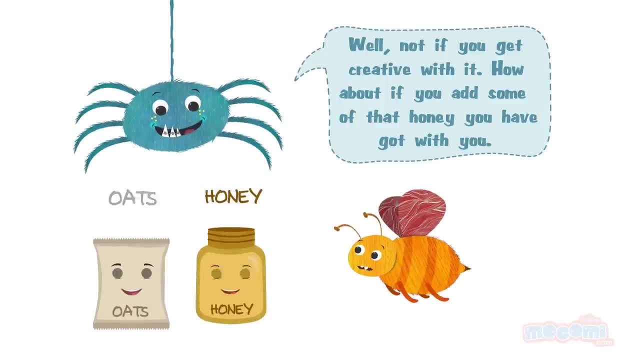 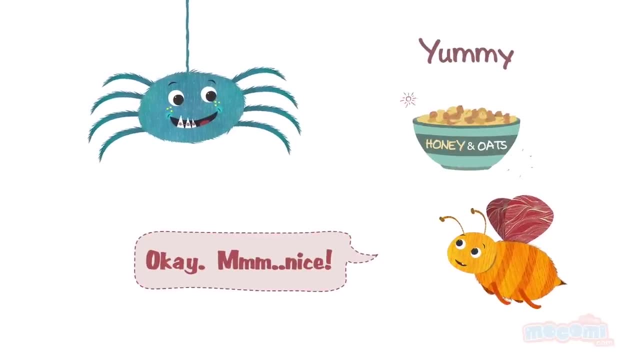 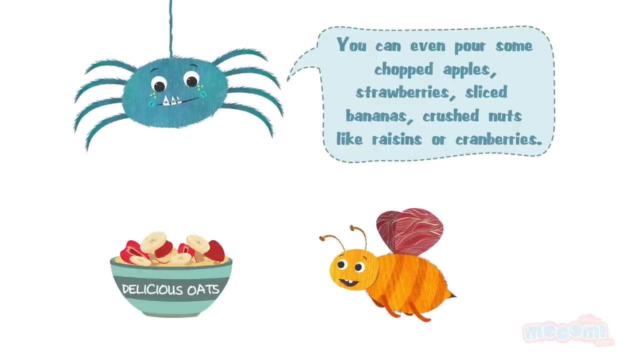 Well, not if you get creative with it. How about if you add some of that honey you have got with you? Okay, Nice, You can even pour some chopped apples, strawberries, sliced bananas, crushed nuts like raisins or cranberries. 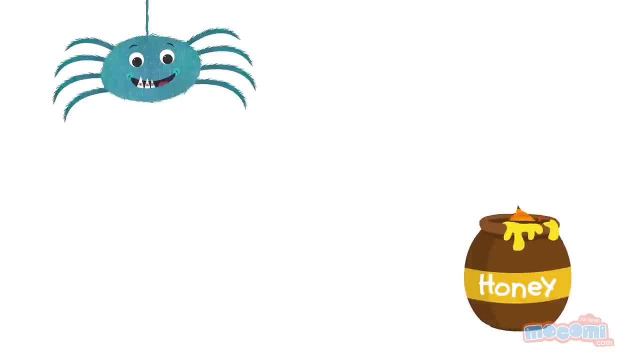 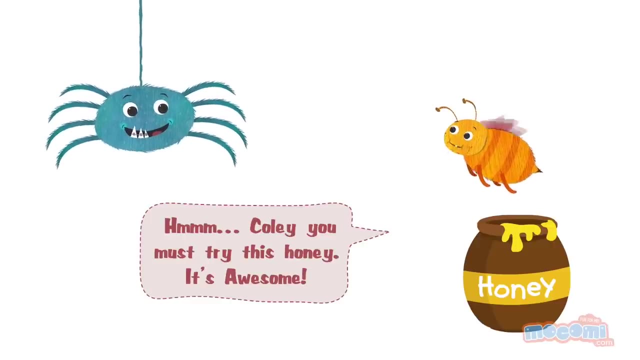 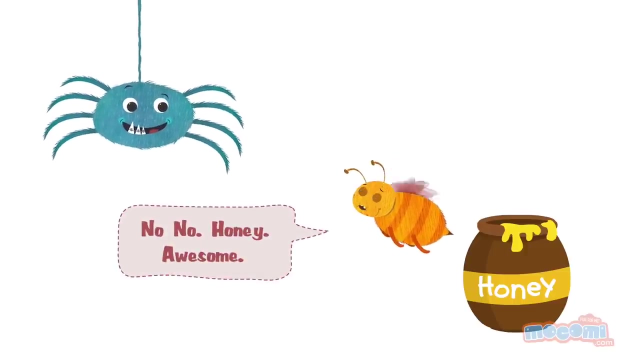 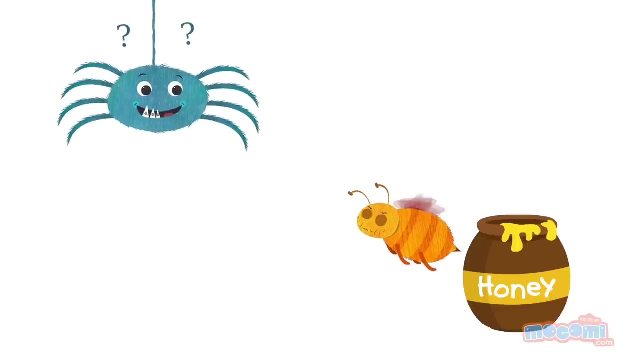 Mmmmm Coley, you must try this honey. It's awesome What? There's a possum in your bunny. No, no, Honey, Awesome. You want money. You shouldn't talk with your mouth full Bumbley. 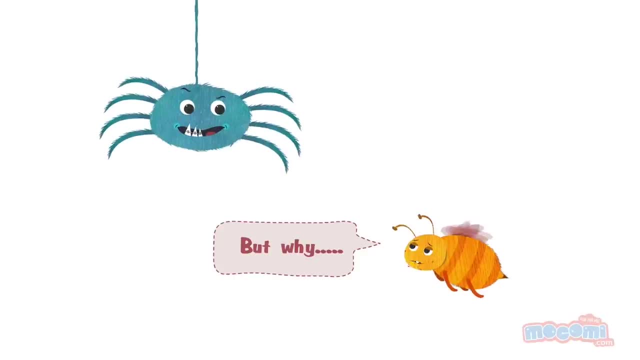 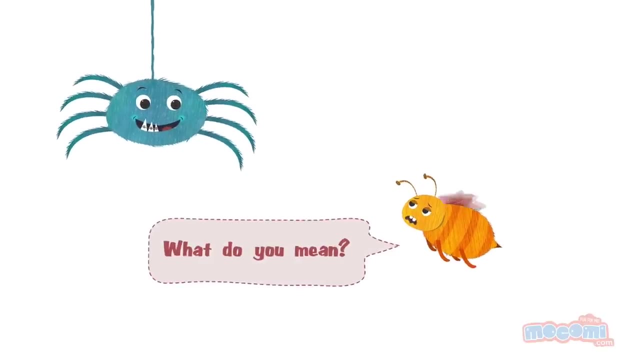 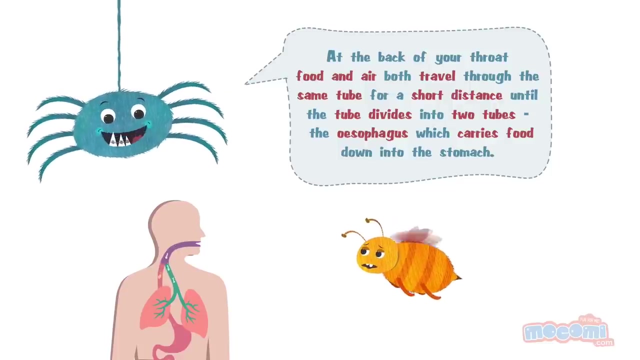 That's why The food has gone down the wrong pipe. What do you mean At the back of your throat? food and air both travel to the same tube for a short distance, until the tube divides into two tubes: The Oesophagus, which carries food down into the stomach. 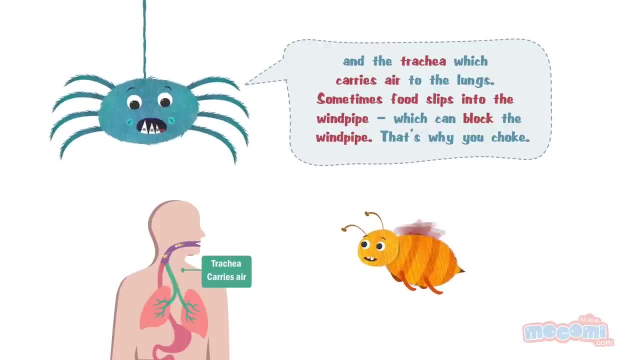 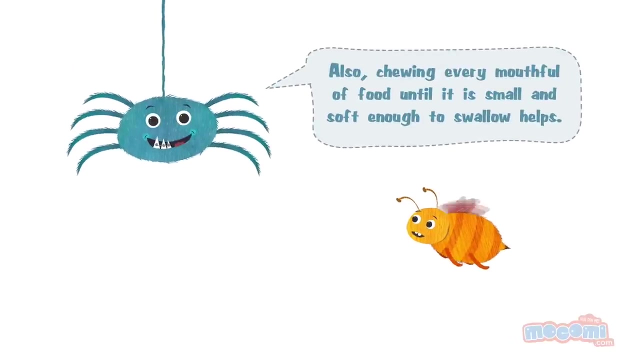 And the Trachea, which carries air to the lungs. Sometimes food slips into the windpipe, which can block the windpipe. That's why you choke Sounds complicated. Also, chewing every mouthful of food until it is small and soft enough to swallow helps. 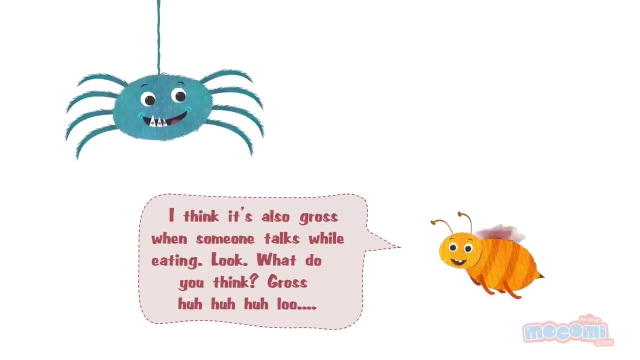 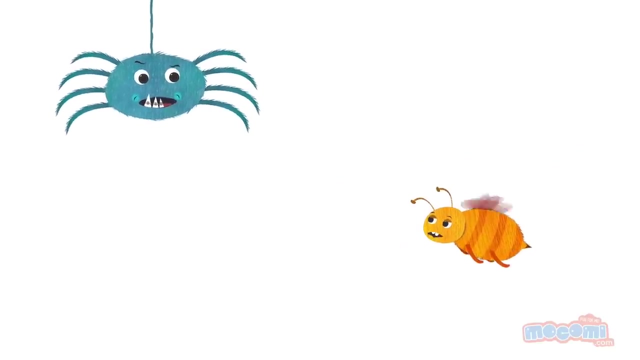 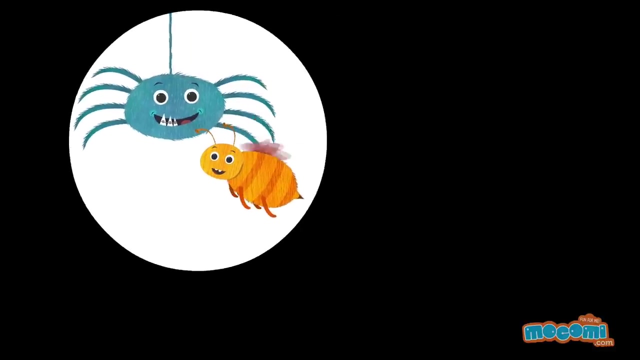 I think it's also gross when someone talks while eating. Look What do you think Gross? huh, No, Some people never learn. Why don't you study? I want a lesson or two, Okay? Okay, I'll read one of thoseга. 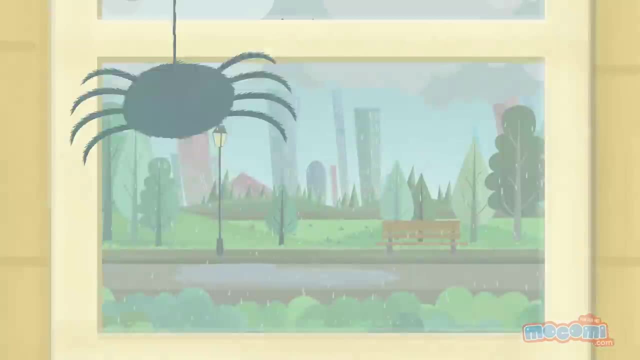 Where's the teacher? Oh, I'm in my room. Oh, I'm in my room. You're up early today. You'll get lucky. Thank you, Daddy. you've been a teacher since I was little. Let's try to get there soon. 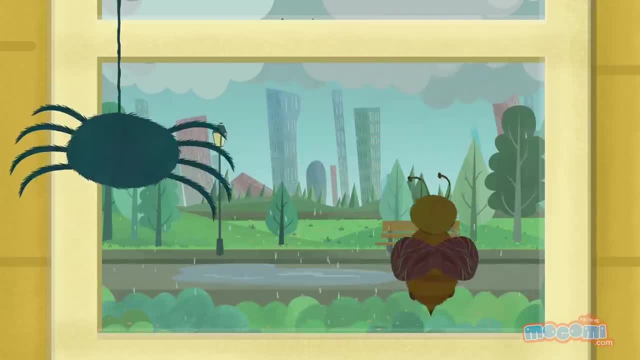 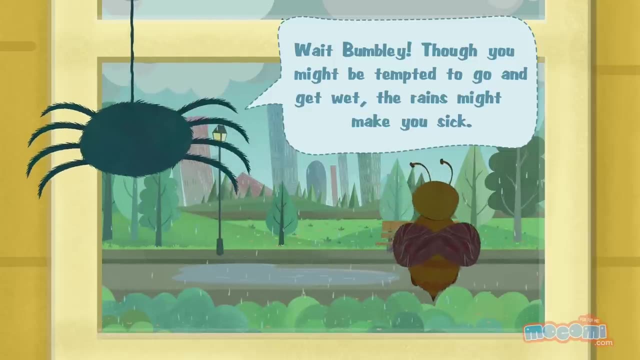 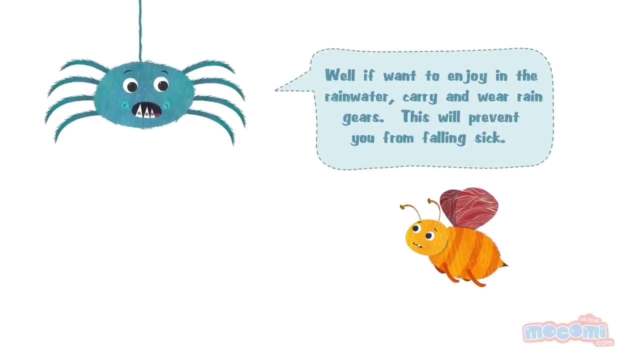 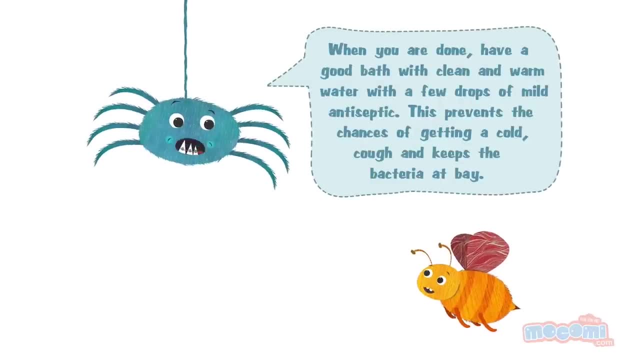 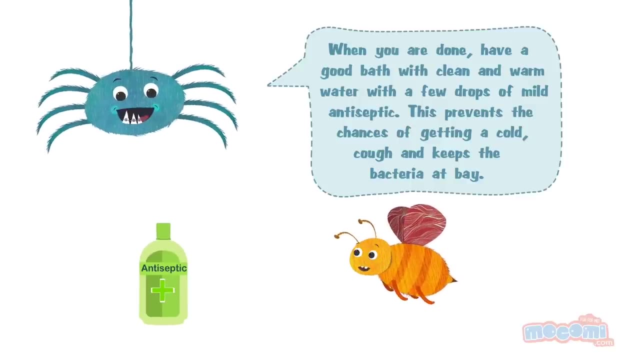 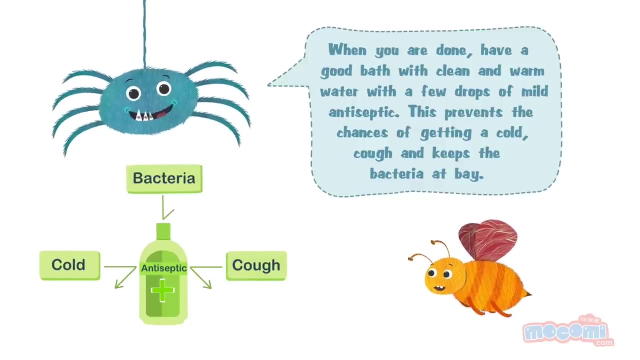 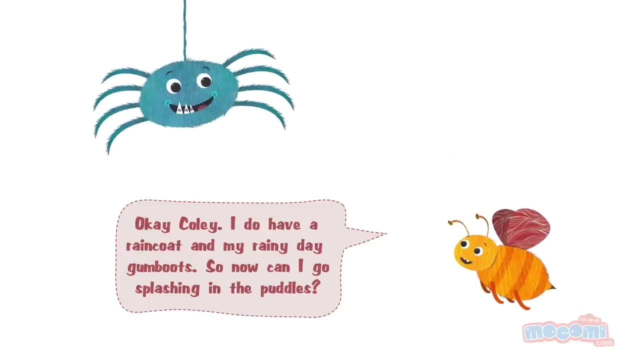 This will prevent you from falling sick. When you are done, have a good bath with clean and warm water with a few drops of mild antiseptic. This prevents the chances of getting a cold cough and keeps the bacteria at bay. Ok, Kohli, I do have a rain coat and my rainy day gumboots. 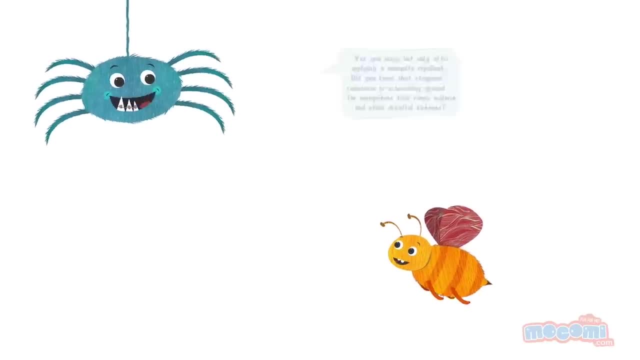 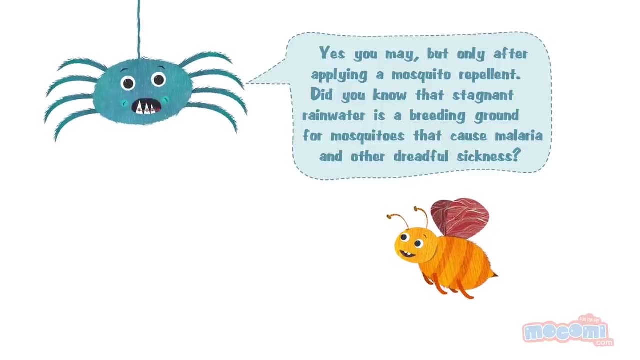 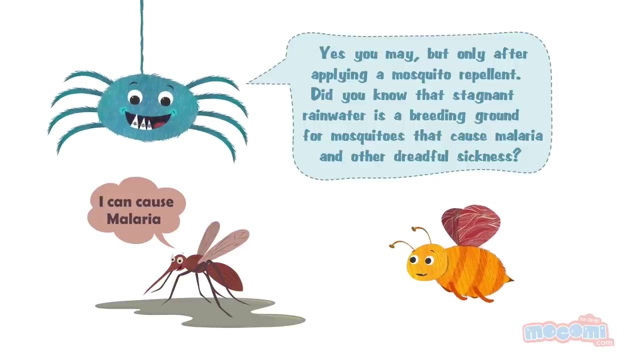 So now can I go splashing in the puddles? Yes, you may, but only after applying a mosquito repellent. Did you know that stagnant rain water is a breeding ground for mosquitoes that cause malaria and other dreadful sicknesses? Nooooooooo. In this season, eye infections are the most common. 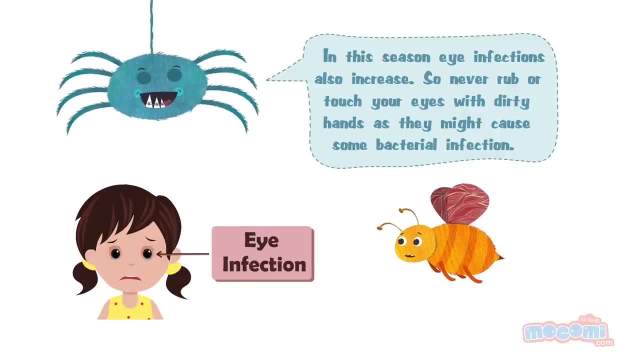 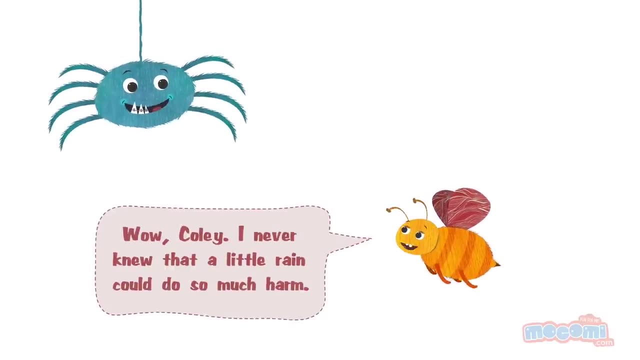 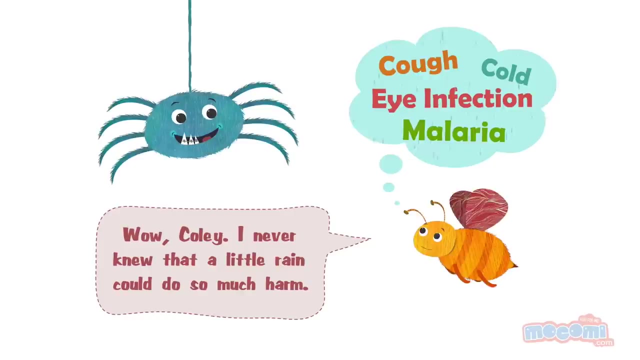 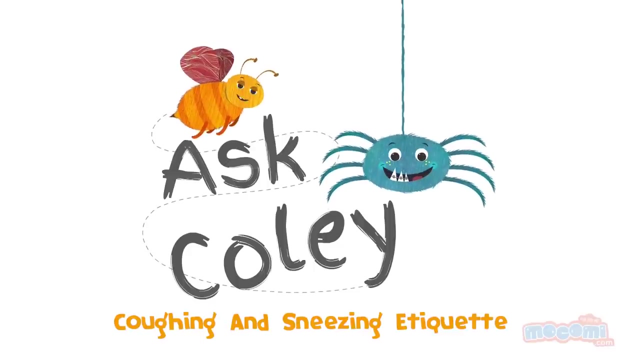 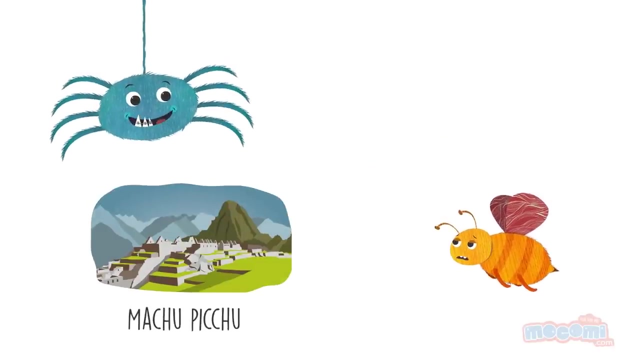 Infections also increase, So never rub or touch your eyes with dirty hands, as they might cause some bacterial infection. Wow, Kohli, I never knew that a little rain could do so much harm. Achoo, You're going too much Upichu. 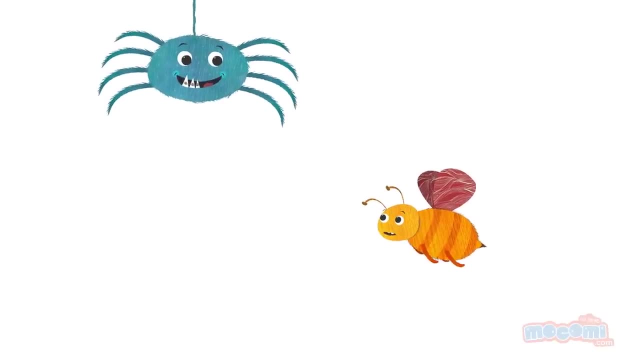 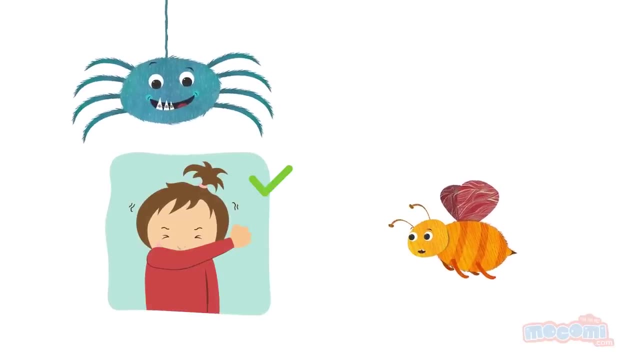 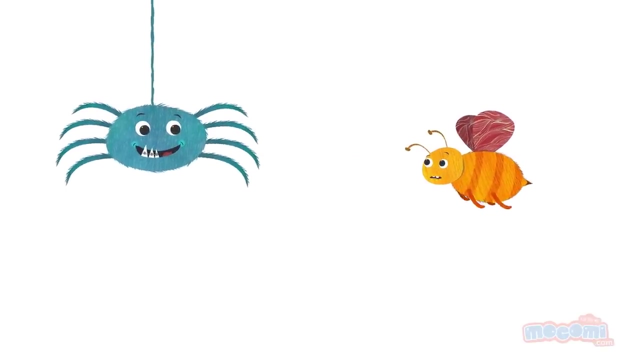 No, That's just me sneezing. Ewww, That's terrible. Haven't you heard Cough and sneeze Elbows? please? What? Why would I sneeze into my elbows when I can sneeze into my hands? 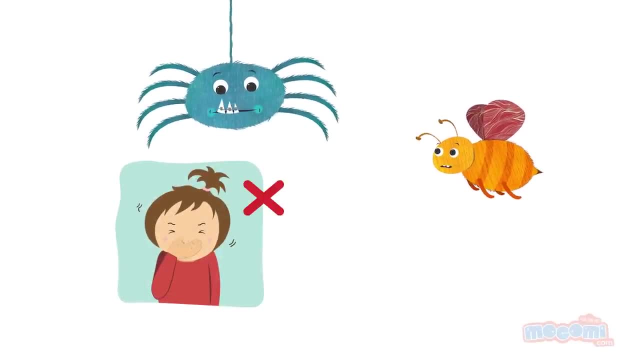 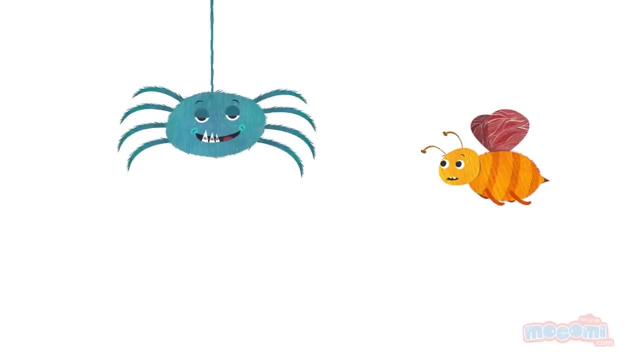 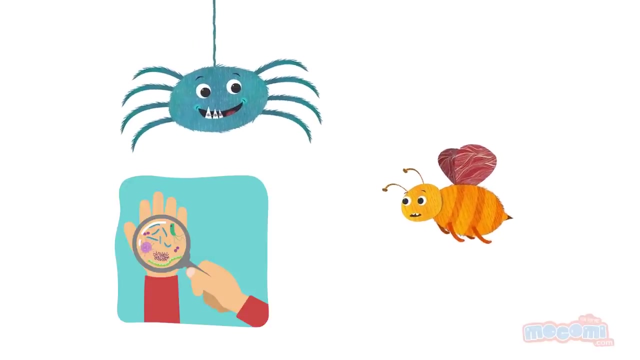 Because that is the easiest way to spread the germs. I thought covering your mouth would help prevent the spreading of the germs. Yes, but what happens after that? What about the things you would touch after that? I hadn't thought of that. 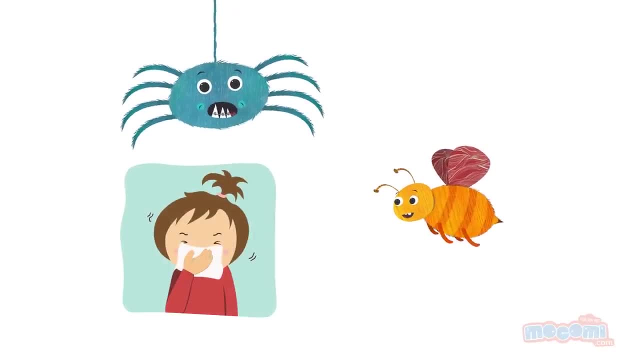 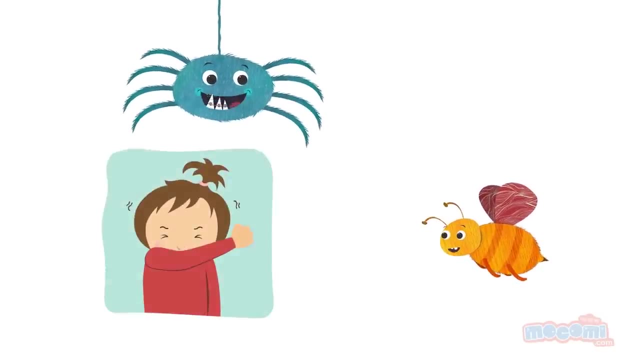 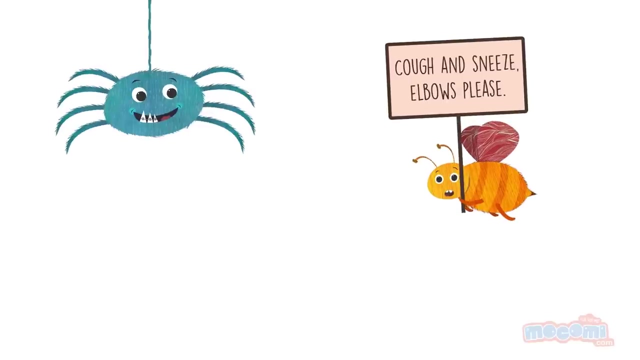 Ideally you should use a tissue when you cough or sneeze And wash your hands later. But if you don't have a tissue, then make sure you use your elbow to cover your mouth And later wash your elbow, Cough and sneeze elbows, please. I shall remember that Also, if you are in a crowd of people, cough or sneeze downwards to avoid sneezing directly at someone's face. I will remember that too When I go to Machu Picchu. Are you sneezing again? 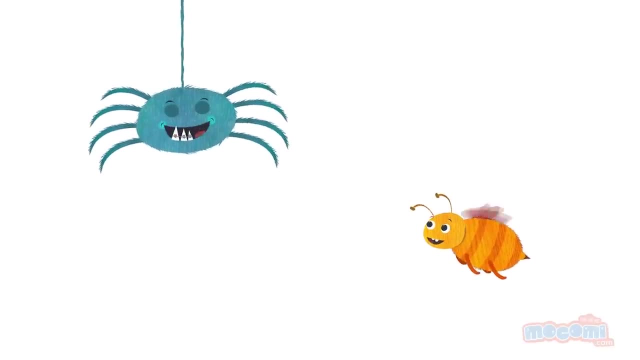 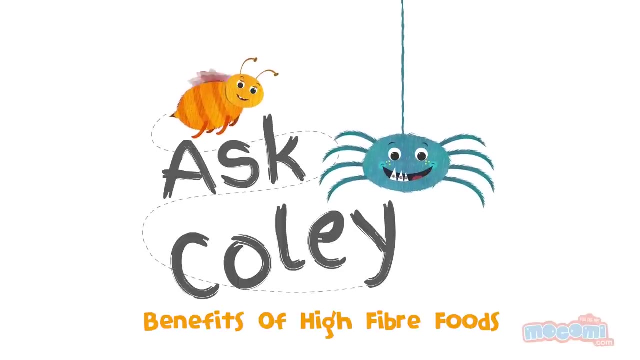 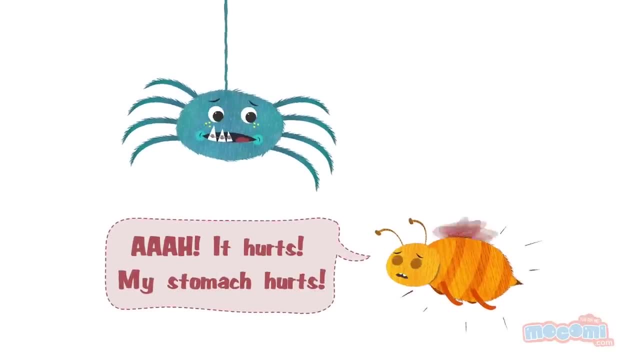 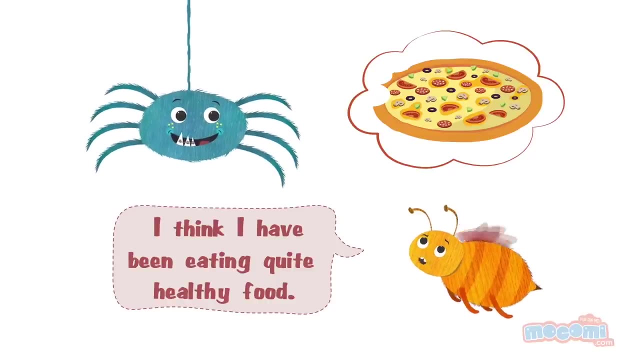 Achoo, Achoo, Choo, Achoo, Choo. Ahh, It hurts, My stomach hurts. What did you eat? now, I think I have been eating quite healthy food. Really, Have you been eating enough fibre? 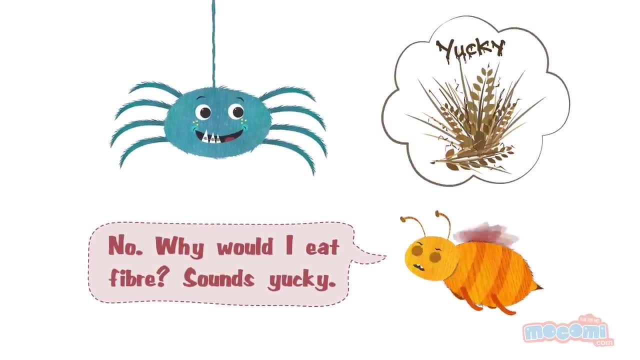 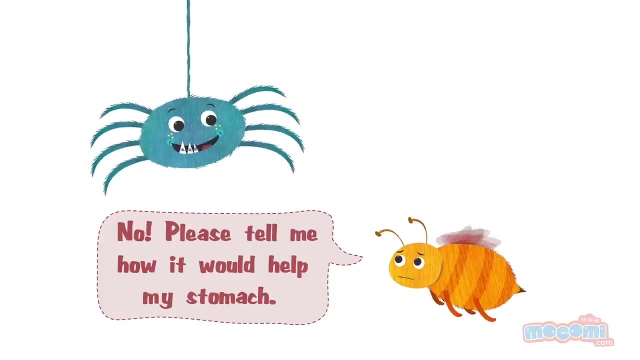 No, Why would I eat fibre? Sounds yucky. Okay then, All the best with your pain. No, Please tell me how it would help me. Please tell me how it would help me. Please tell me how it can stop my pain. 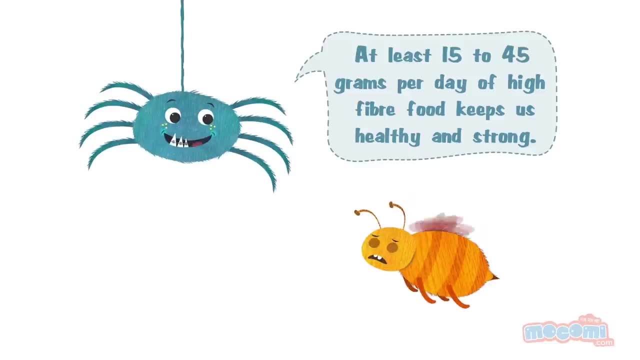 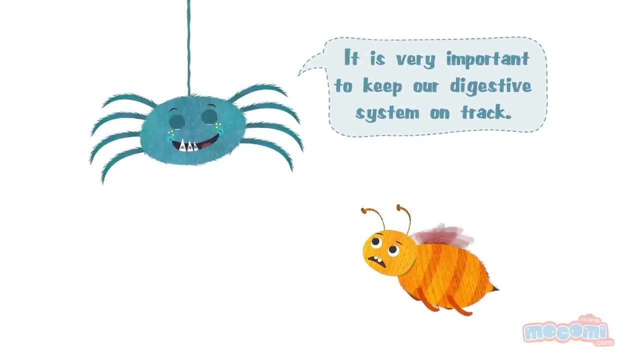 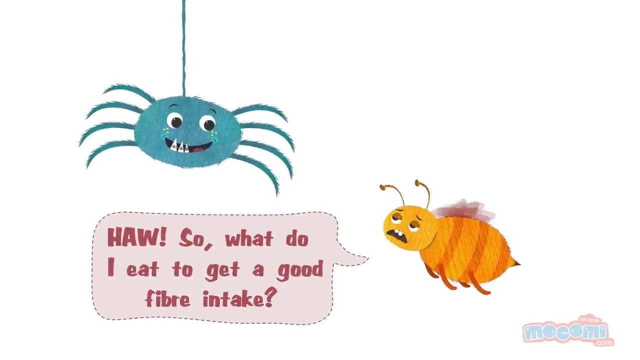 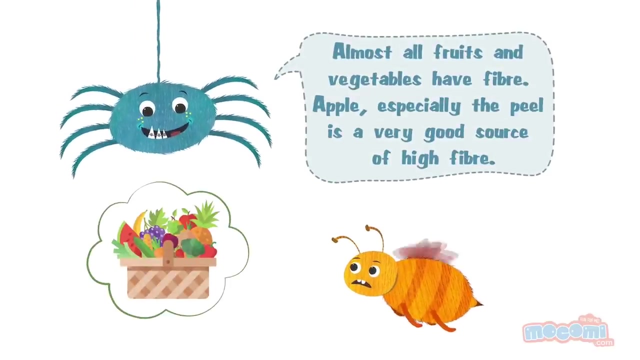 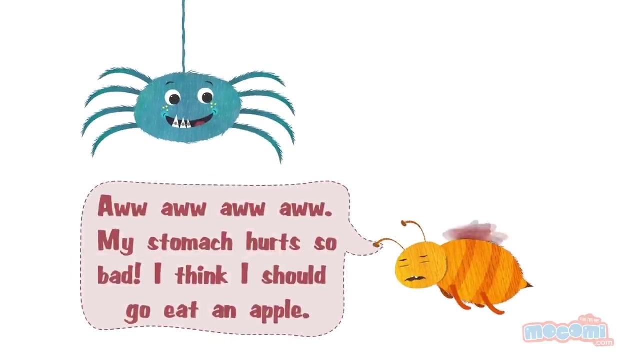 my stomach. at least 15 to 45 grams per day of high fiber food keeps us healthy and strong. it is very important to keep our digestive system on track, huh. so what do I eat to get a good fiber intake? almost all fruits and vegetables have fiber. apple, especially the peel, is a very good source of high fiber. my 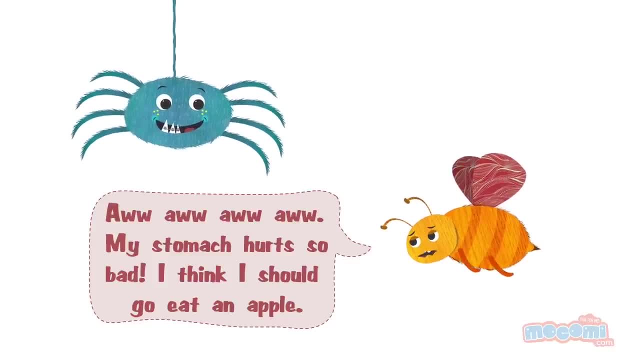 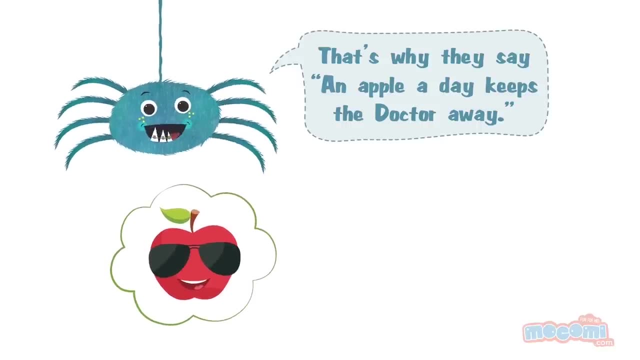 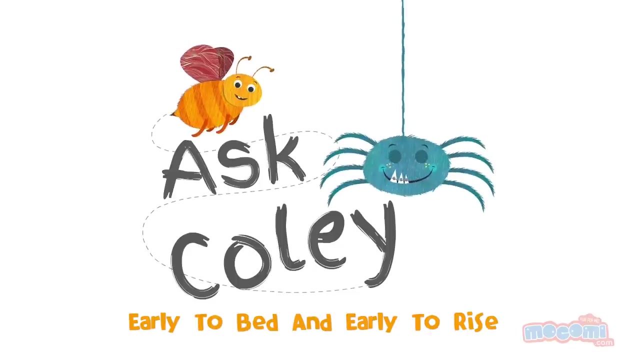 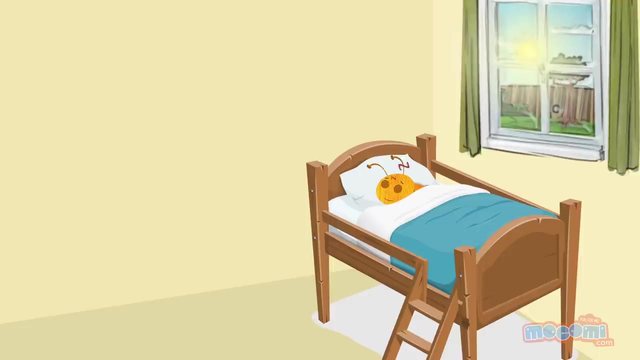 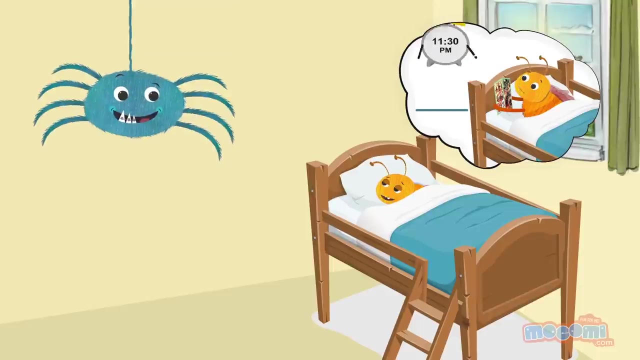 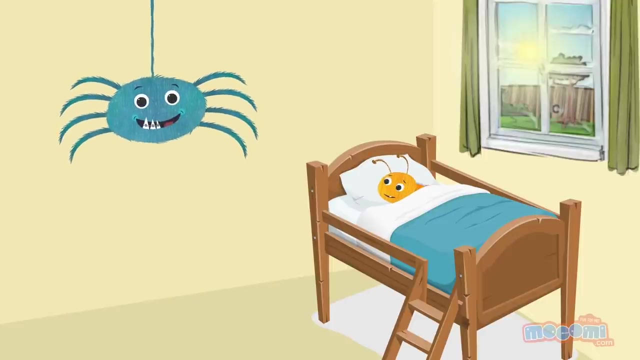 stomach hurts so bad I think I should go eat an apple. that's what they say. an apple a day keeps the doctor away. oh golly, let me sleep some more. I slept a little late last night, but this happens every night. you always sleep late and then you do not want to wake up in the 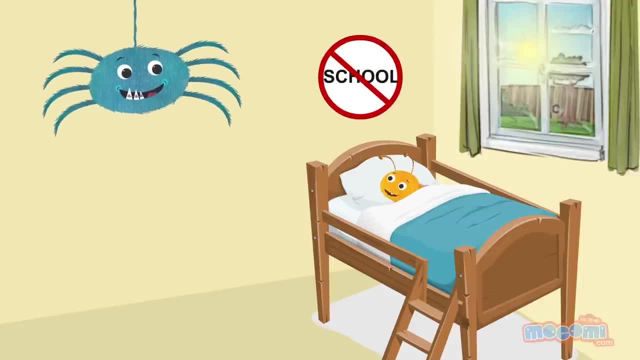 morning. why should I wake up in the morning early? I have no school today, so let me sleep. even if I get up now, I will be all grumpy. yes, going late to bed and waking up late makes you grumpy. if you want to be happier, fitter, healthy and smart, then you need to go to bed early. and wake up early. how will that make me smarter? when you wake up? you need to wake up early and you need to go to bed early. when you sleep early, it benefits your body emotionally, physically and helps in the cognitive development of your brain cells. the growth hormones work between: 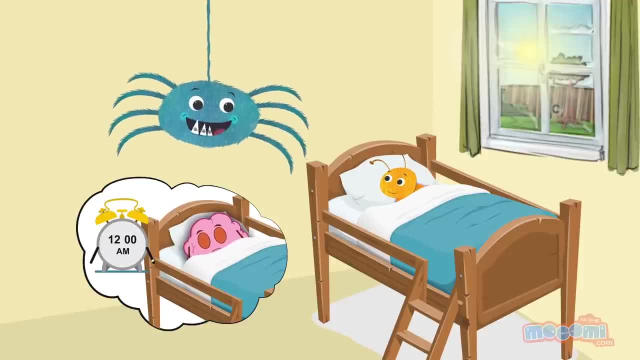 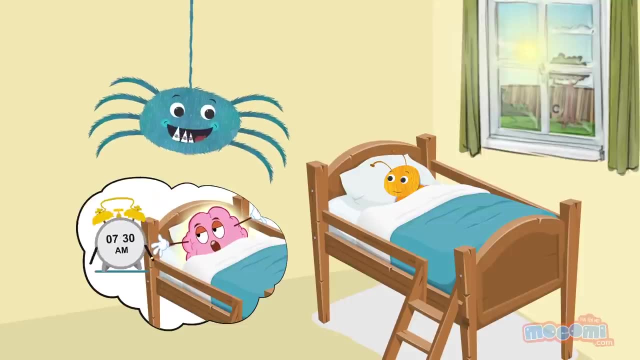 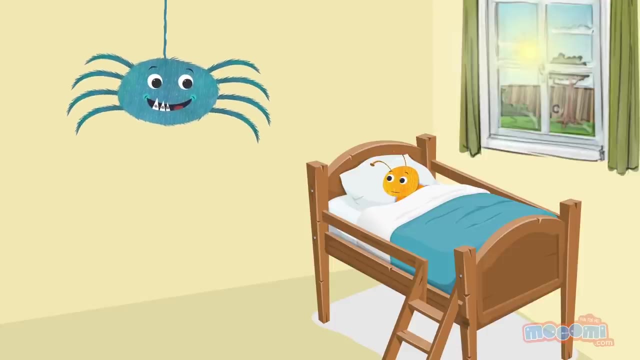 9 and midnight and help you grow faster and better. when you complete 8 hours of sleep, you wake up early and fresh, not groggy and grumpy like now. I get a. yes, the same. early to bed and early to rise makes a man healthy, welly and wise. 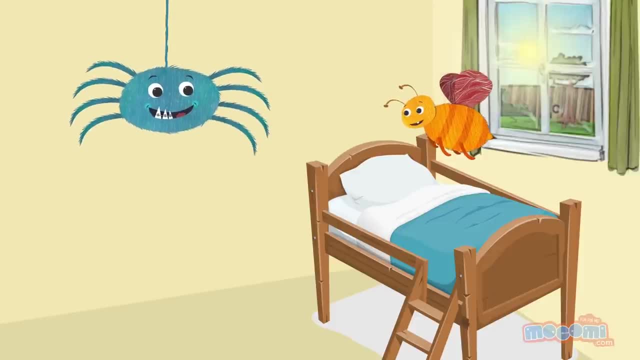 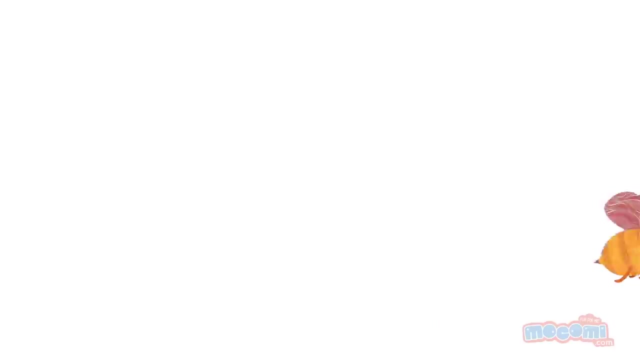 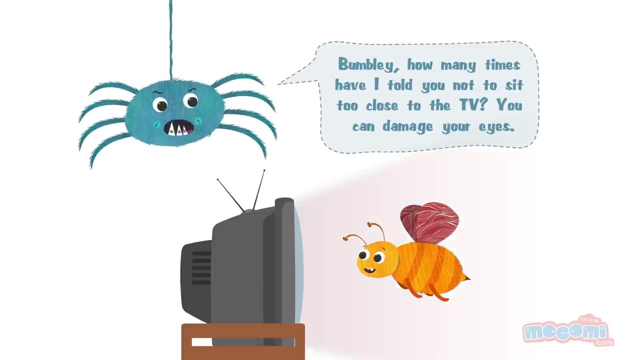 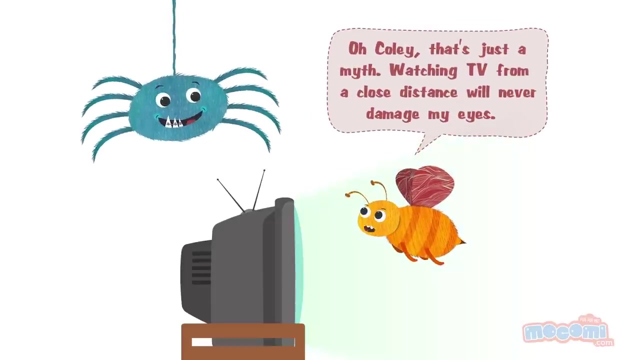 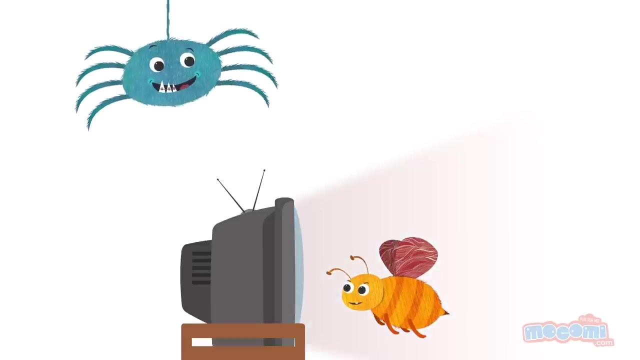 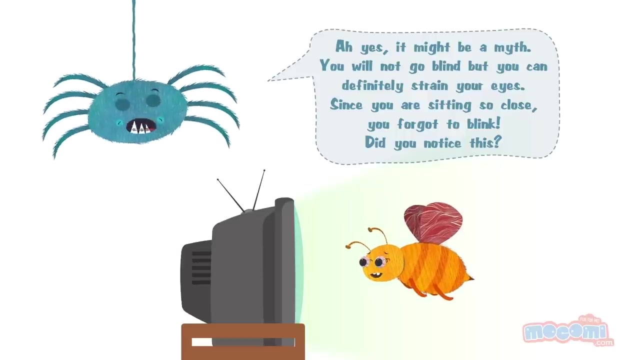 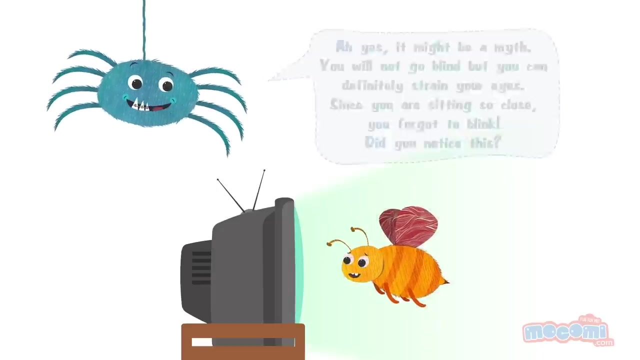 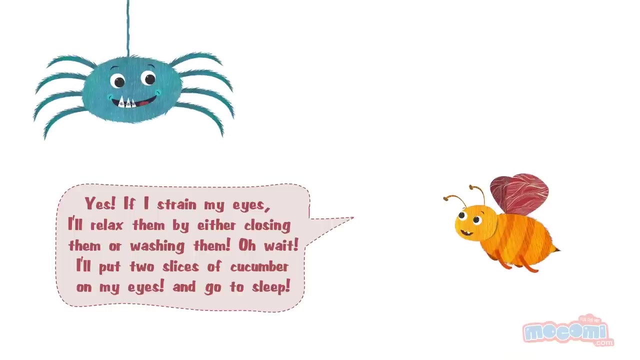 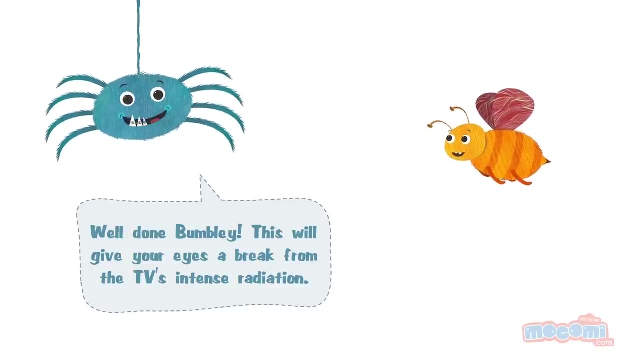 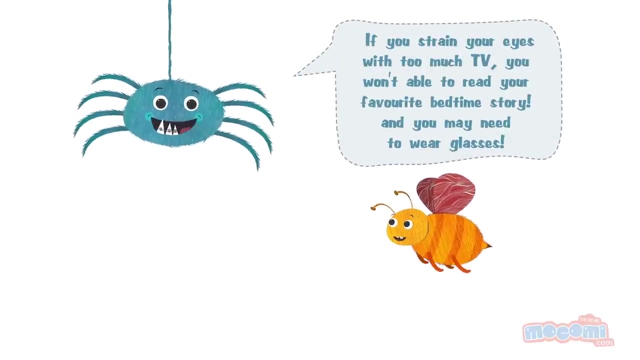 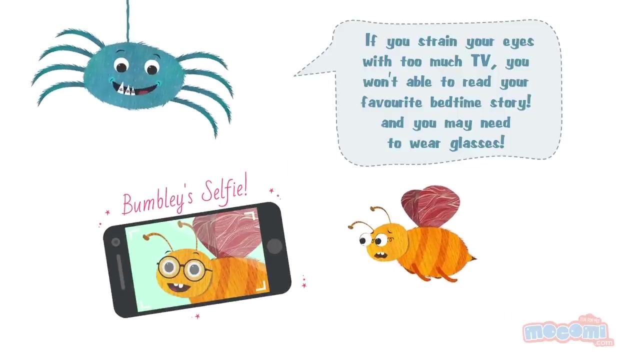 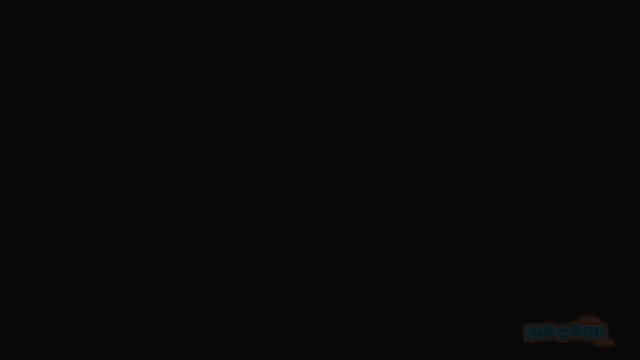 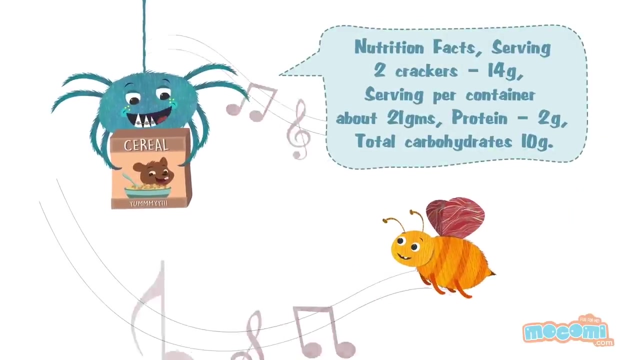 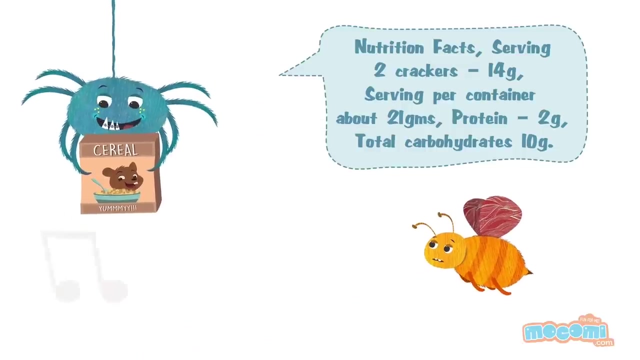 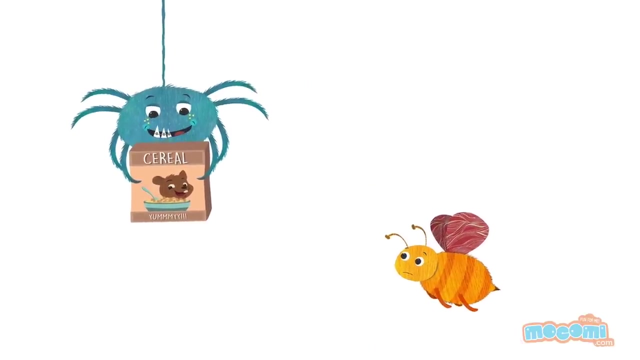 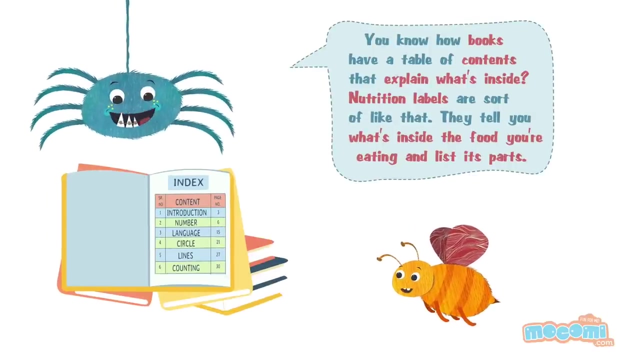 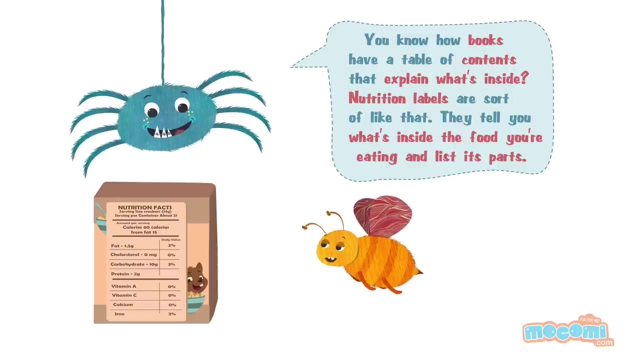 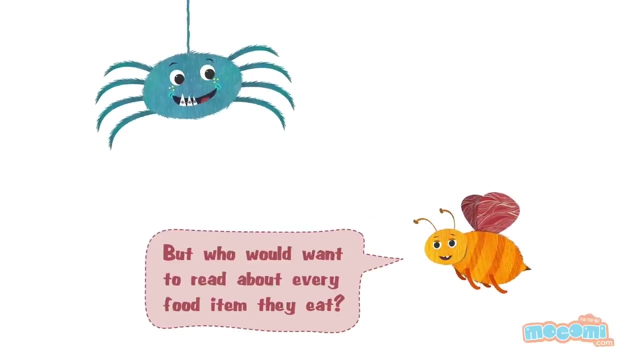 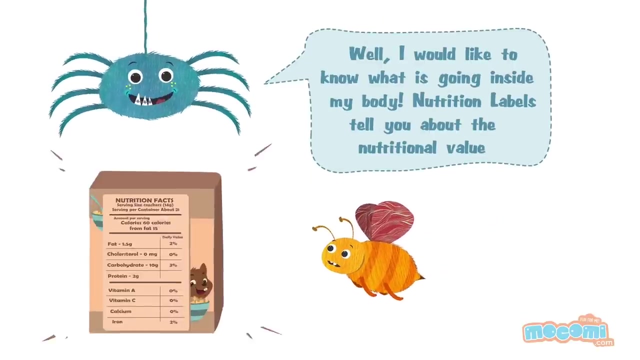 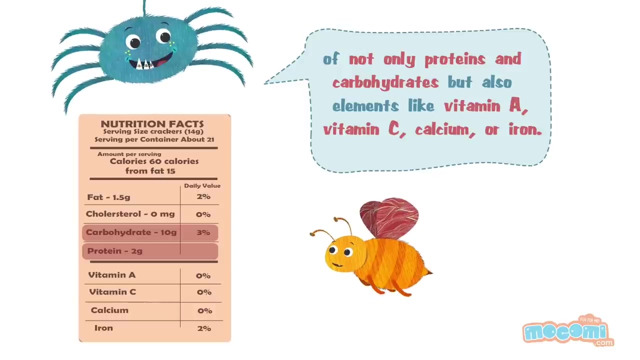 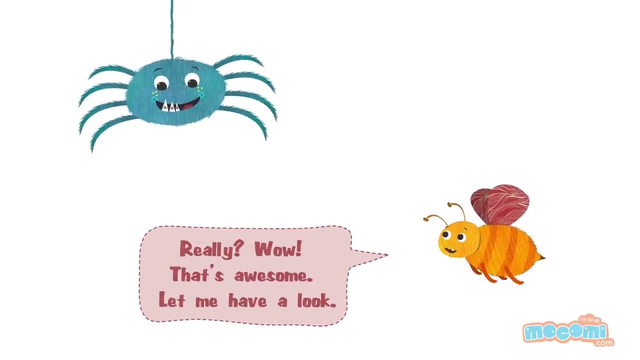 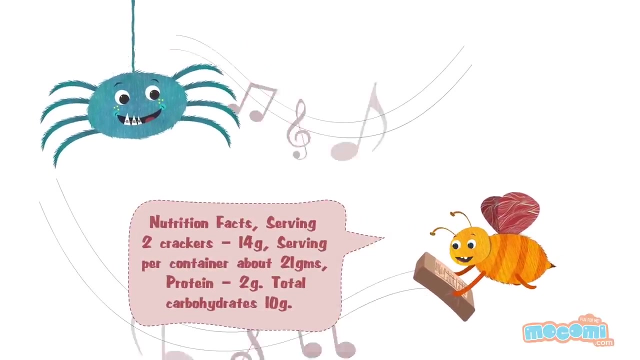 must be true. I'll try and change my habits, Coley. that's great, and I will help you to do that. you, the nutrition labels tell you about the nutritional value of not only proteins and carbohydrates, but also elements like vitamin A, vitamin C, calcium or iron. really, wow, that's awesome. let me have a look. nutrition facts serving to crackers. 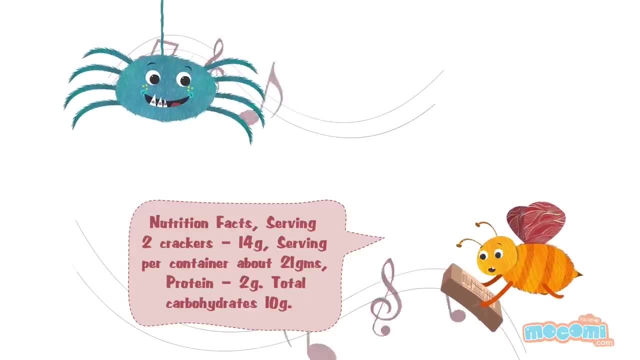 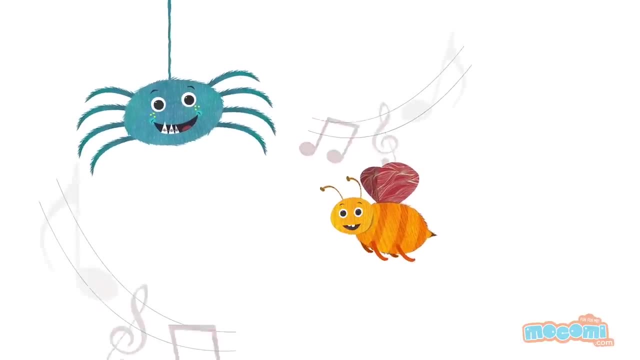 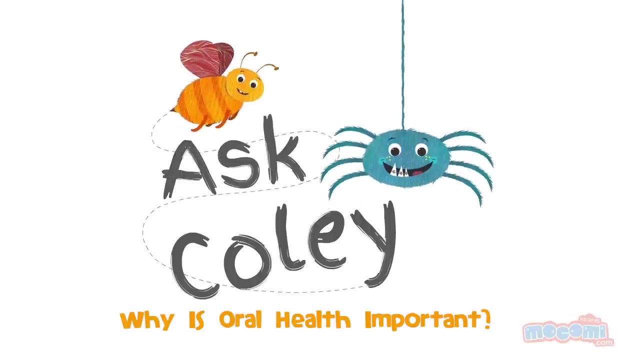 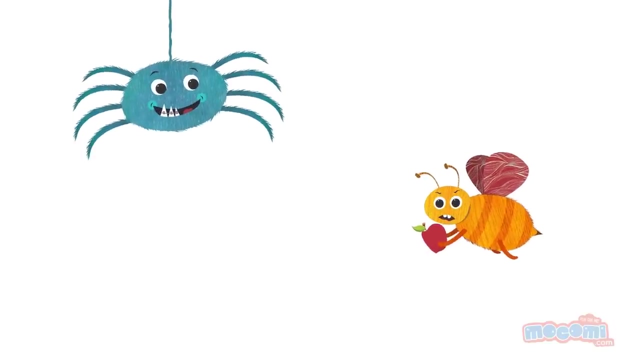 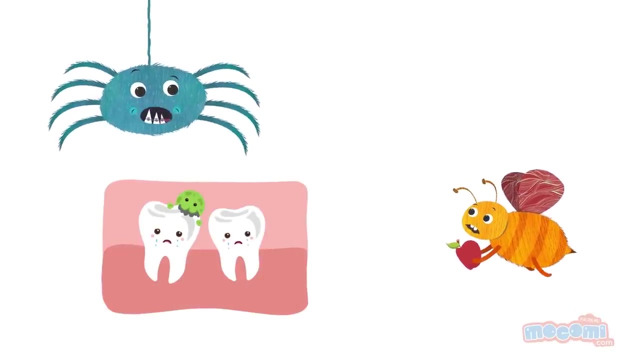 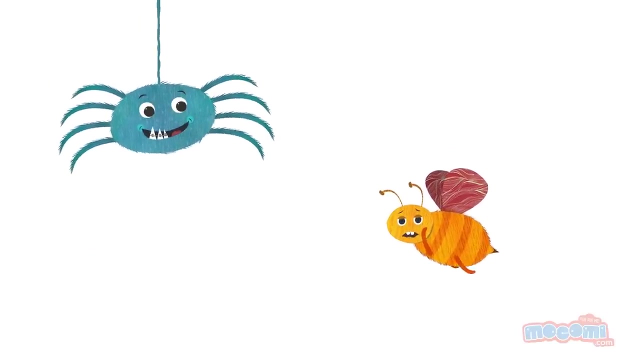 14 grand serving per container. now you got it. ouch, ouch, it is a bad apple. it is so hard, are you okay, mom Lee? it is a soft apple. are your teeth or gums all right? oh, my teeth do hurt, that is because you do not take care of them. bumbley well I. 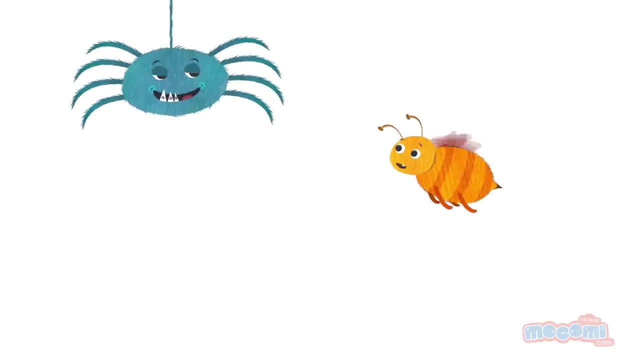 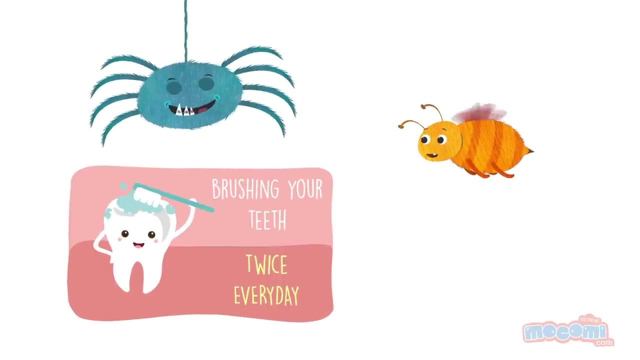 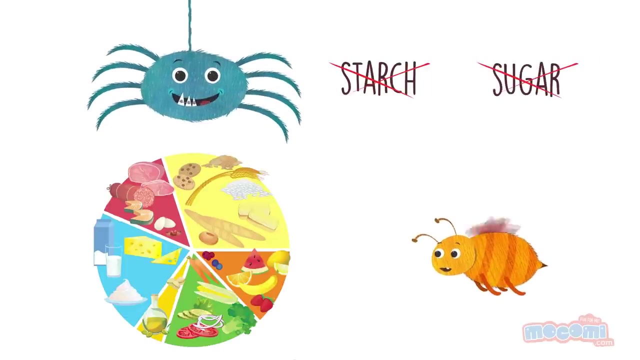 do brush every day, sometimes even twice. you are so funny, bumbly. a good oral healthcare involves more than that. like what like for a start, brushing your feet twice every day like eating a well-done plate of peanuts. I like eating the best well balanced diet that is not too starchy or sugary, which causes tooth. 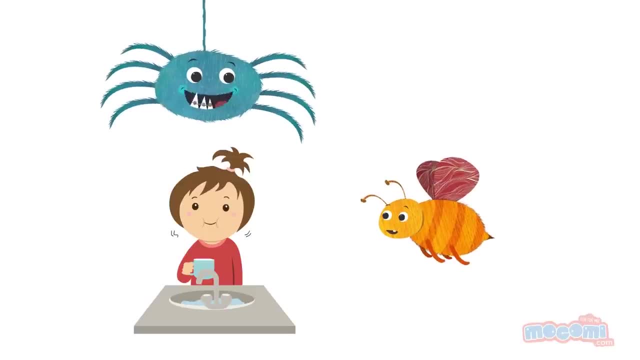 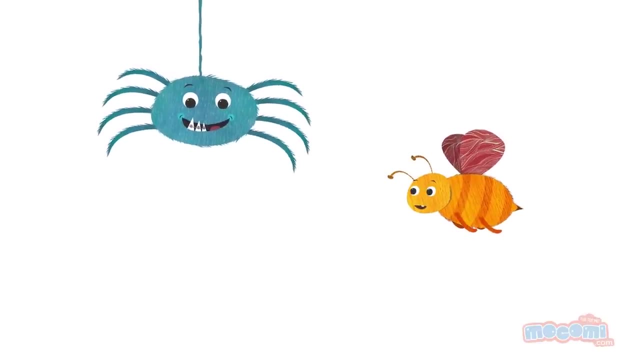 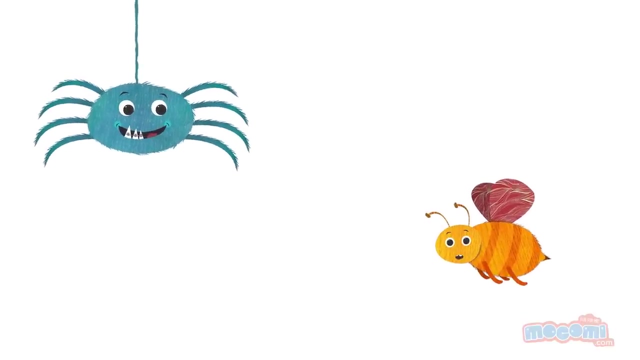 decay. also, rinse your mouth after every meal so that nothing is stuck in your teeth. drink plenty of water and pay regular visits to your dentists. these are one of the easiest things to do. yeah, and you will be thankful for it all your life. I do like the idea of being able to eat chocolates all my life and yes, 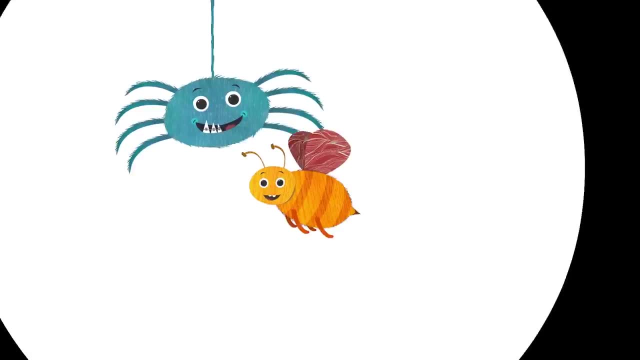 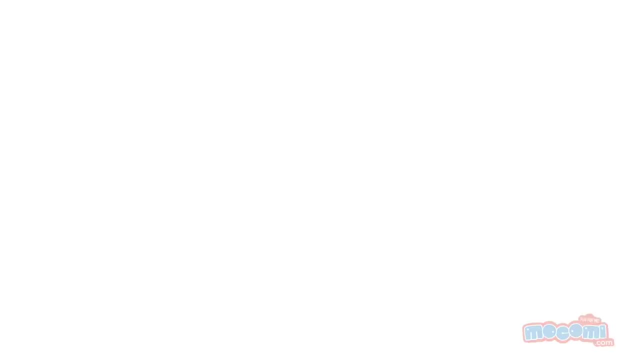 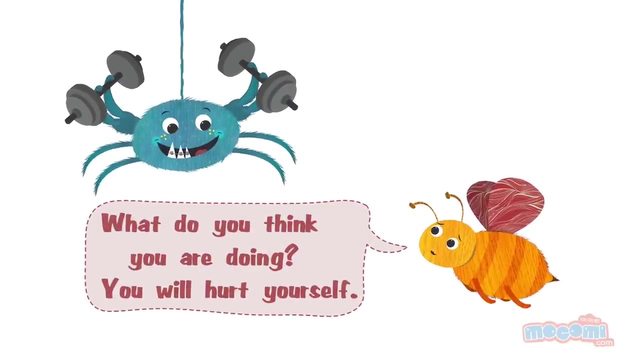 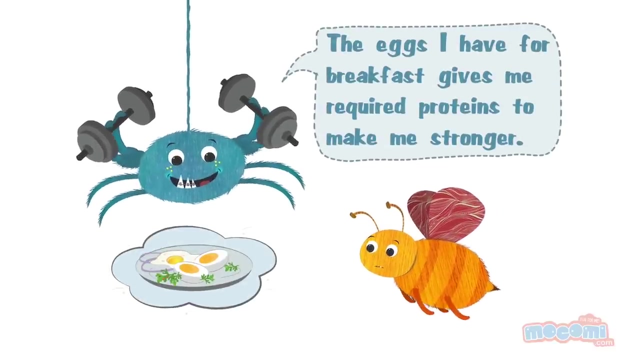 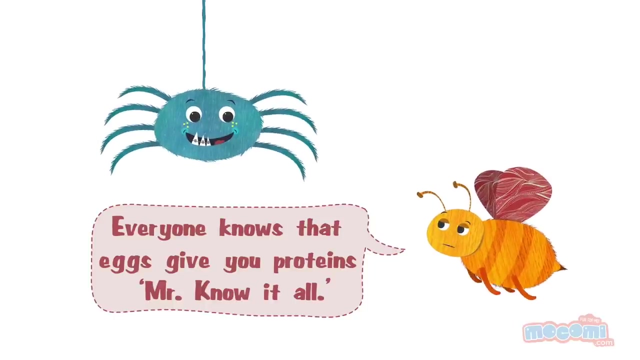 yes, and apples and grapes. what do you think you are doing? you will hurt yourself. I'm strong enough untuk nahn. i am strong enough to have chocolate or not. The eggs I have for breakfast gives me the required proteins to make me stronger. Everyone knows that eggs give you proteins, Mr Know-it-all. 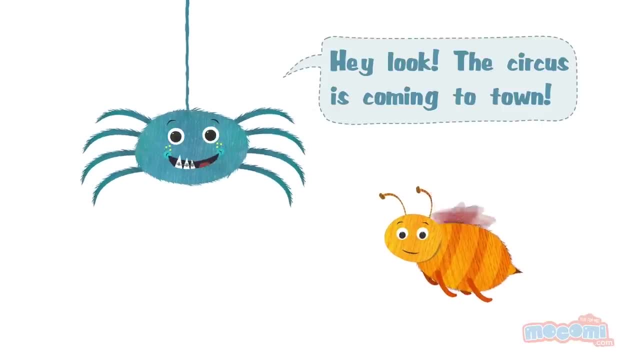 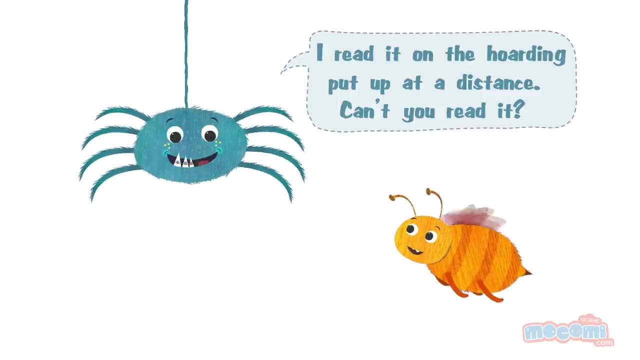 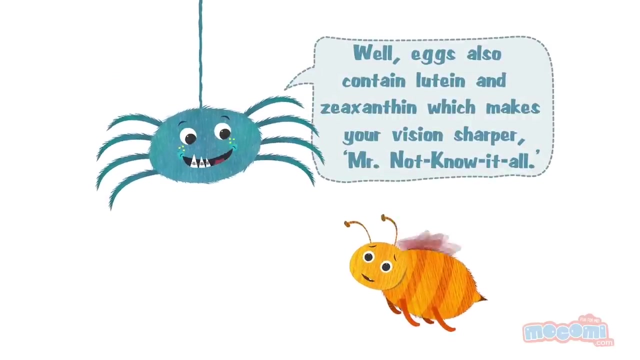 Hey look, The circus is coming to town. How do you know? I read it on the hoarding, put up at a distance. Can't you read it Where? No, I can't. Well, eggs also contain lutein and zeaxanthin, which make your vision sharper.